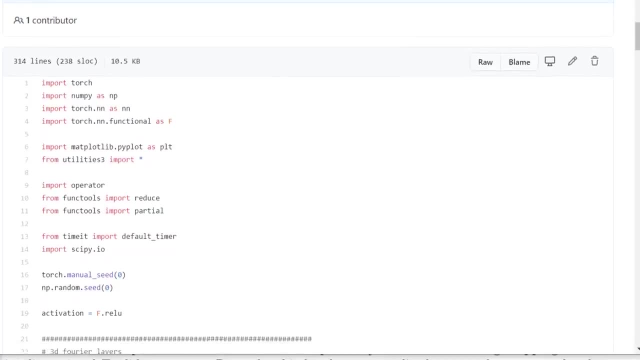 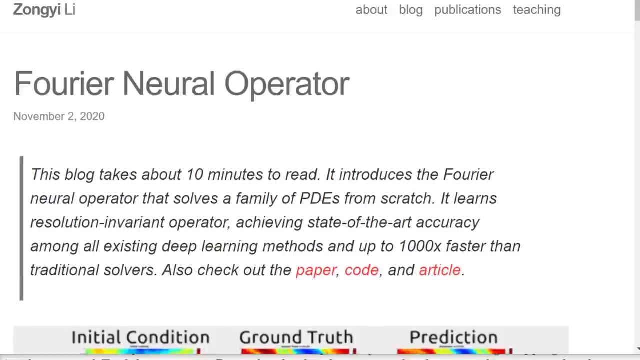 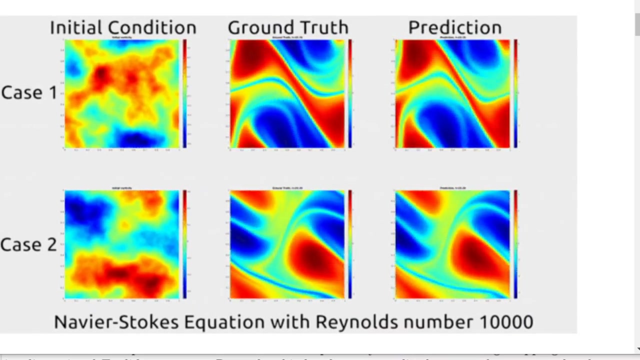 we'll get into the code a little bit as well, because I think it helps to understand what's going on. And I want to start out by. this is the. the blog post by one of the authors, And it's pretty good to get a basic overview of the paper, And here is the motivational example. So 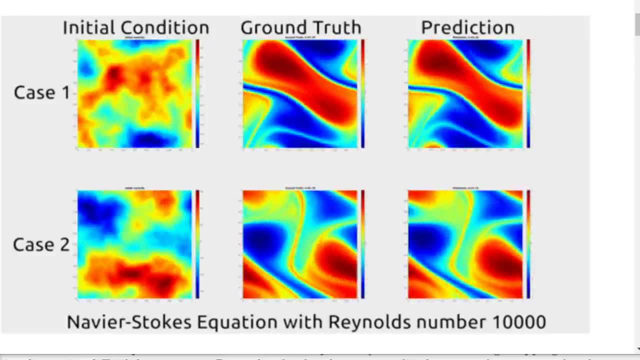 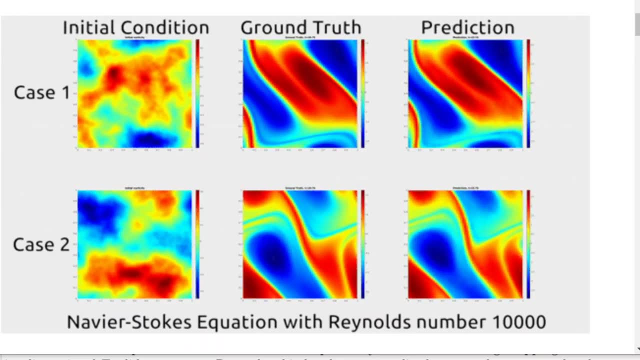 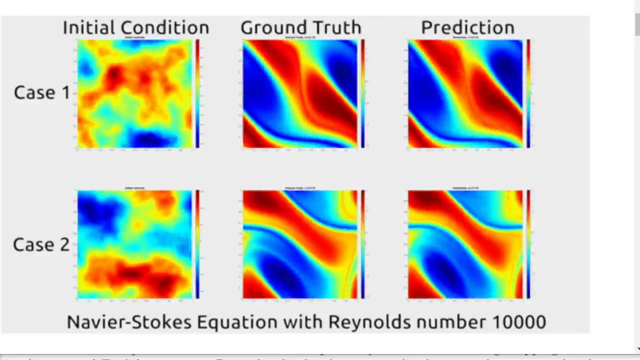 the motivational example is the Navier Stokes equation, which is an equation in fluid dynamics. So you're trying to predict how a fluid evolves over time given a certain parameters, like it's a viscosity and a forcing function, So basically how sticky it is and how hard you stir it, And then you 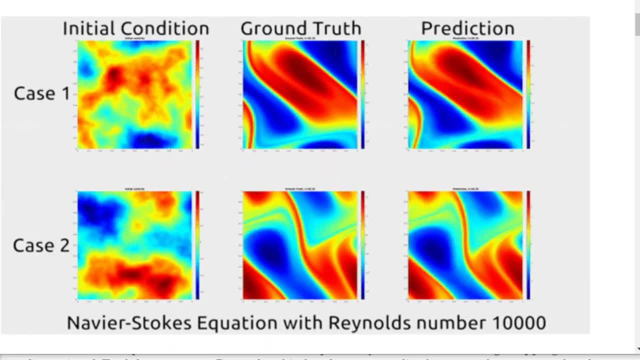 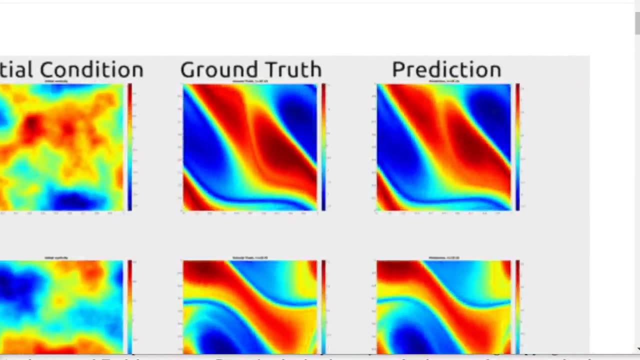 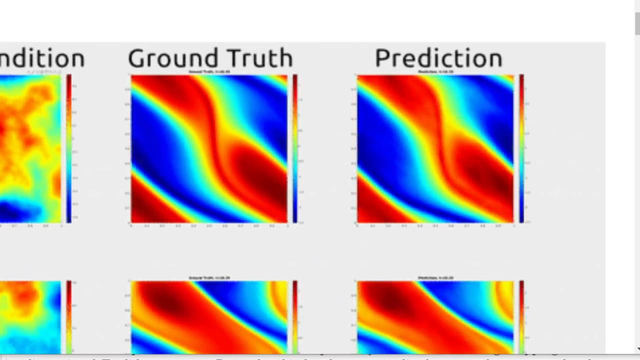 want to know how it evolves over time And you can see, on the left is given an initial condition And I think on the right is sort of a rollout after the 10th time step until the 50th time step And the ground truth is obtained with a sort of classic numerical solver where you do little time steps and 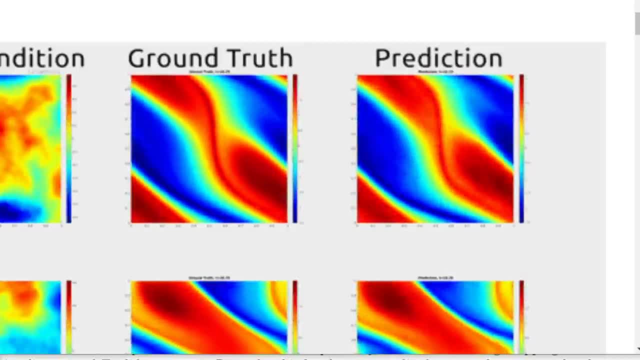 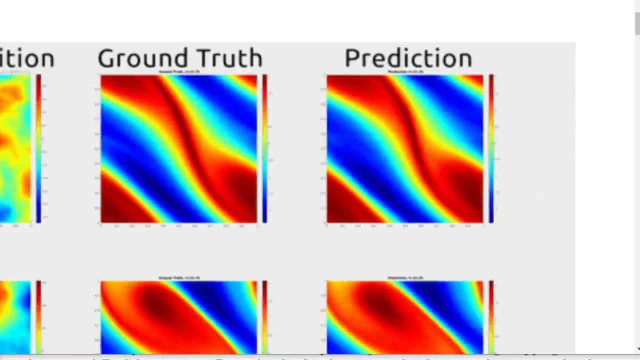 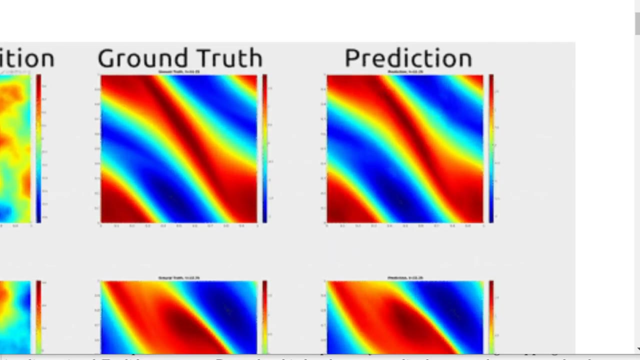 you calculate the interactions And then this takes a lot of time and compute. And on the right is the prediction of this new Fourier neural operator that this paper develops. And you can see it's almost equal And the gist of it is that the thing on the right simply takes one forward. 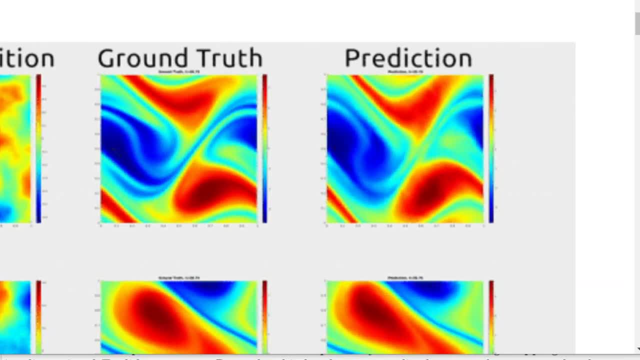 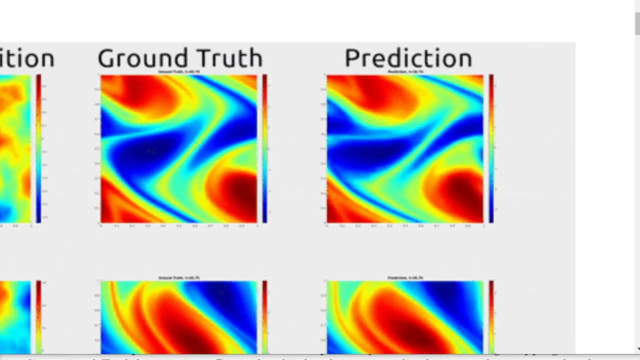 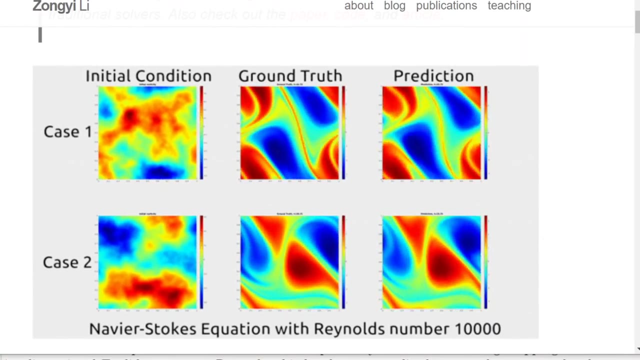 propagation through a neural network. So it takes like super, like point 00, something of a second to compute the thing On the right, whereas the thing on the left is quite hard to compute and, as I understand, can take minutes. So use here you see, the, the motivational example. these things are described by partial 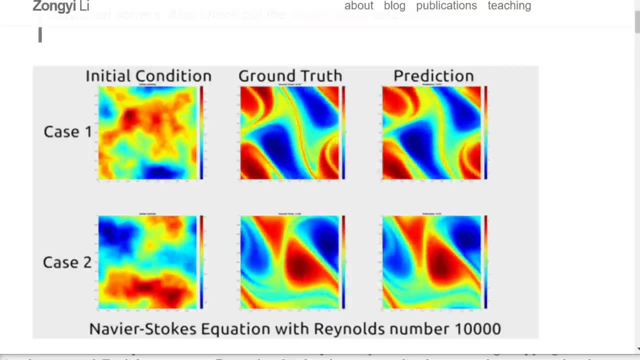 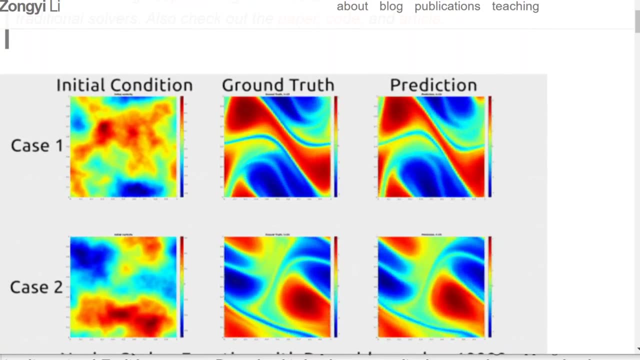 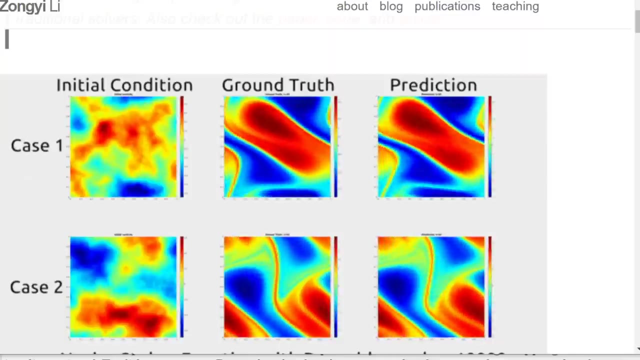 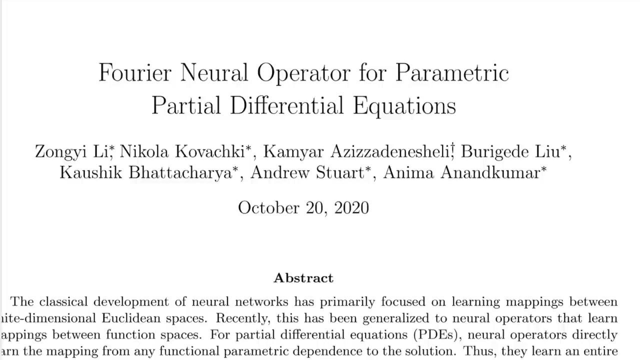 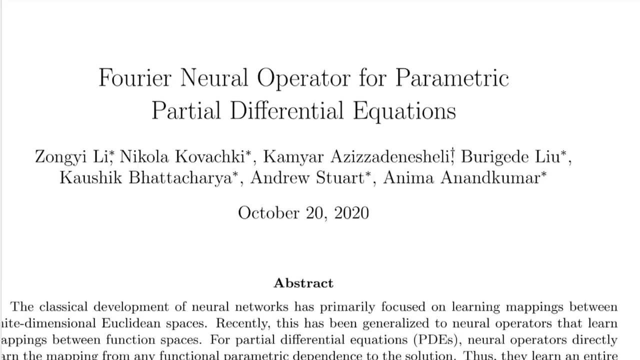 differential equations, which are sort of linearized, linearized ways of describing how the system evolves over one time step, And it'd be cool if we could solve these faster, because this is applications in aerodynamics and other types of engineering fields. All right, so let's jump into the paper And, as always, if you like content like this, consider sharing it out, telling your friends about it and subscribing, of course. So the paper is called Fourier neural operator for parametric partial differential equations And it's by 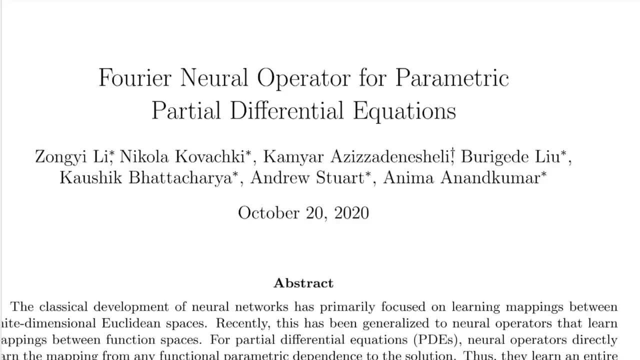 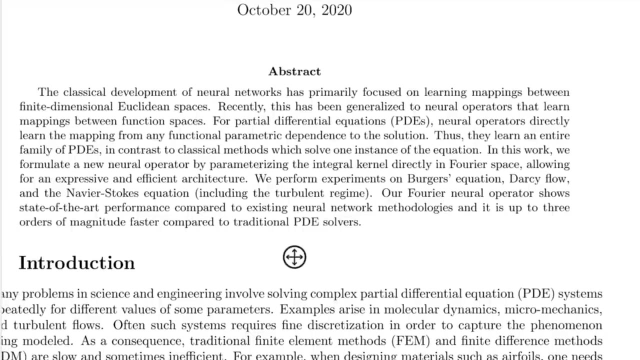 Songyi Li, Nikola Kovachky, Kamyar Aziza Dinesheli, Burigede Liu Kaushik Bhattacharya, Andrew Steward and Anima Anankumar of Caltech and Purdue University. So I feel I feel the paper is both very cool and a bit overhyped. So we're going to see what it does. It's it's for a particular type of PDEs And it has a lot of, let's say, engineering choices that make it possible to solve with neural networks, but also that limit its applicability to where the 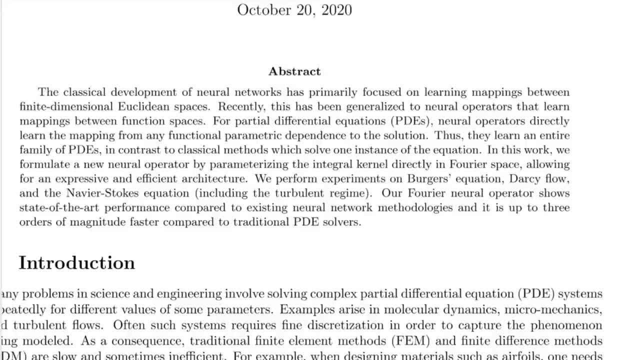 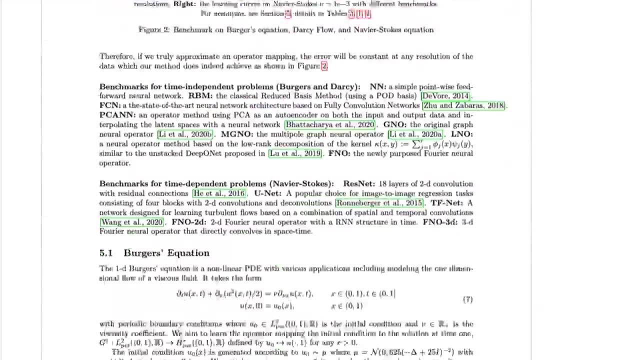 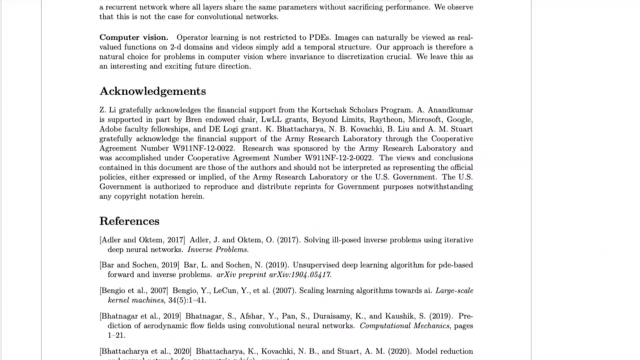 classical methods would be applicable where this thing isn't. So there are trade offs, definitely to reach the sort of speed up that they reach. But we'll get into this First. I actually want to scroll down right here all the way, because there is something that you don't often see in the sort of machine learning field And that is here in the 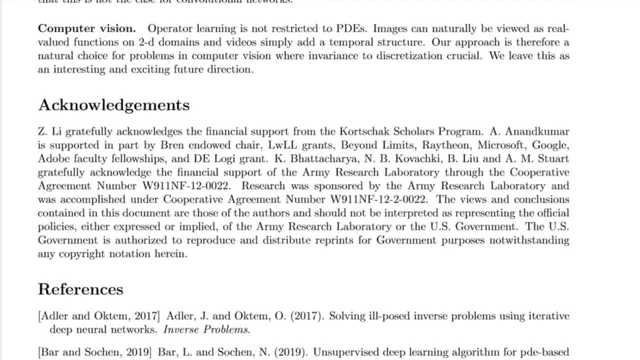 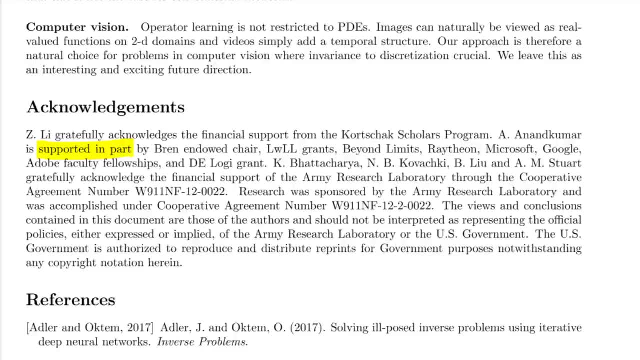 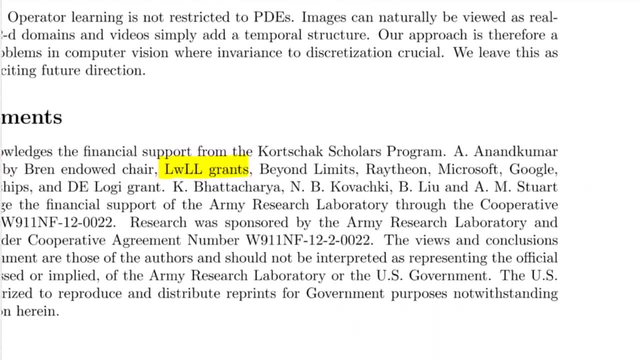 acknowledgments section, And I just, you know, I just find this, I just find it interesting, don't. don't don't regard this as anyone, But here we are supported by the LWLL grants, which I understand is DARPA Beyond Limits, which is like a makes soft or makes AI, or systems for things like gas and oil and so on, with British Petroleum as a main sponsor, Raytheon, which, of course, is a giant military manufacturer. 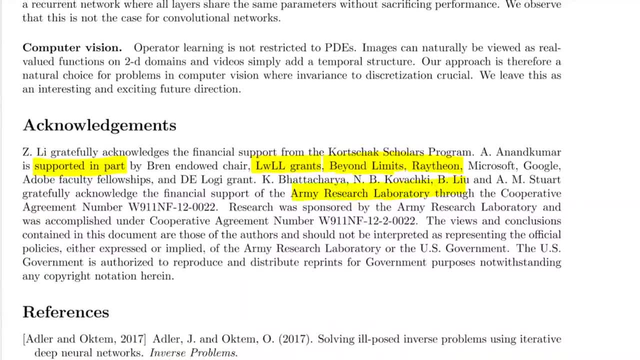 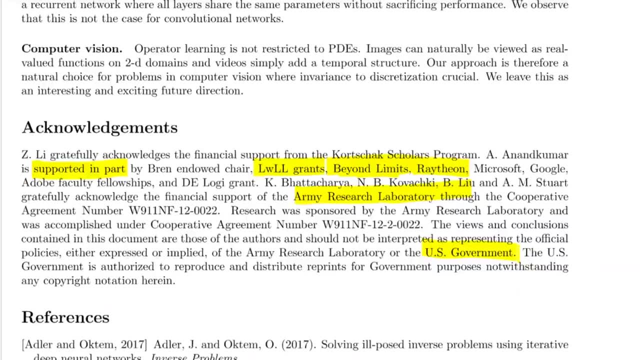 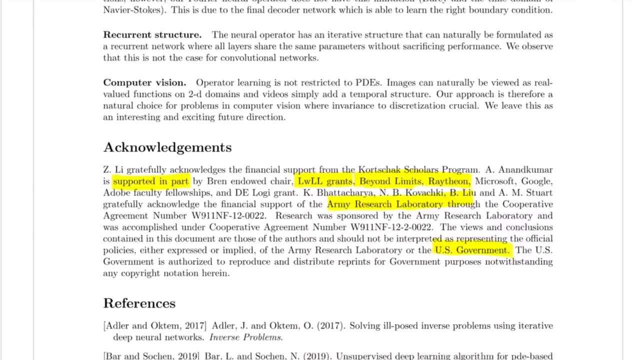 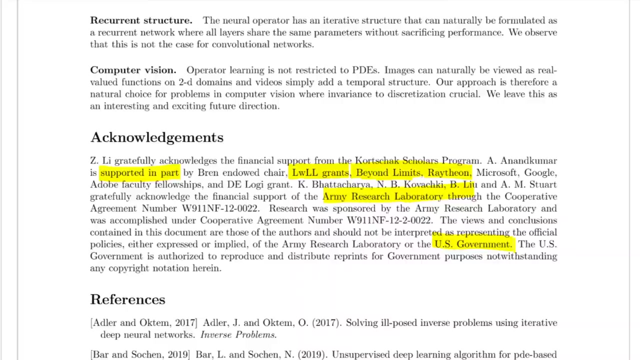 We have the Army Research Laboratory and so on. So so you can see that this, this is kind of- I don't know, I don't see this often. This is sort of a good bouquet of sponsorships. Of course there's also Microsoft, Google and so on. Yeah, but it's just, it's just interesting to see that that the, the army, has pretty heavily into these things, And of course there's also Microsoft, Google and so on. 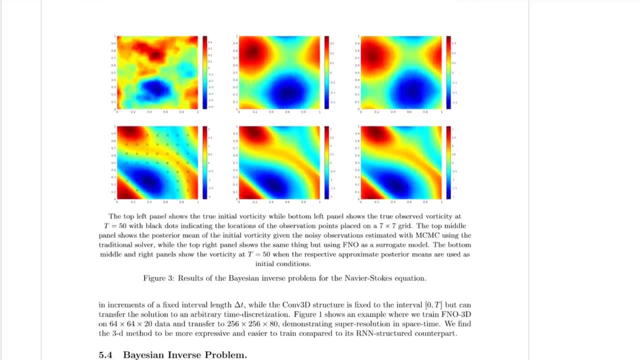 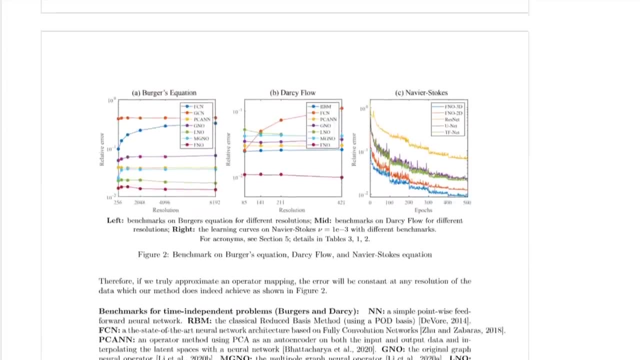 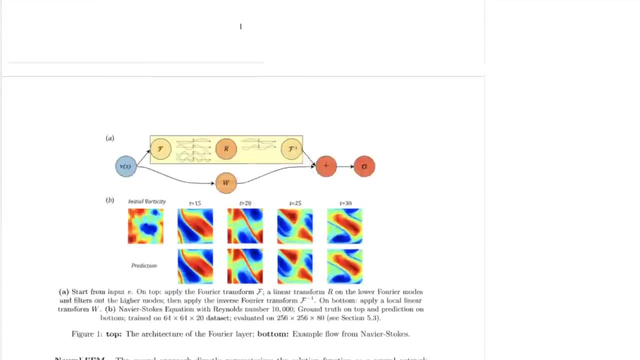 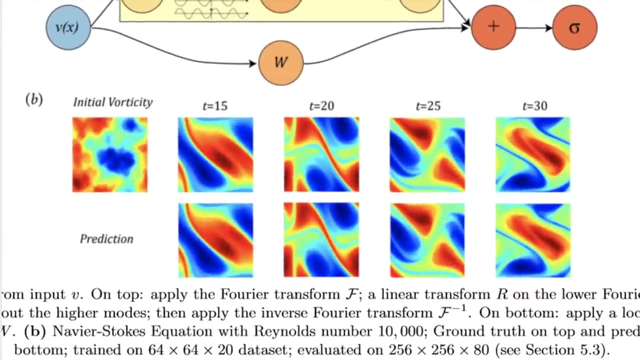 they would be. I mean, rockets need to fly and they need to be aerodynamic, and so on. So yeah, I'm not saying this is bad or good, I just thought it was. it was interesting that you know Raytheon would would be a sponsor of this. All right, so let's dive in. As we said, we're interested in these types of of problems. right here, where you have this thing called, so the, there's this quantity called. 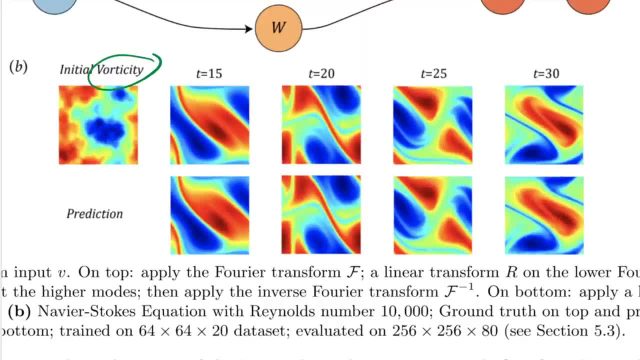 the vorticity which, as I understand, is a derivation of the viscosity. So it sort of tells you how the fluid is is moving right now And so this, this state right here, and then you apply a sort of constant forcing function And you want to know how that evolves over time So you can see at time, step 15, you get sort of this picture. So these, these move past each other. 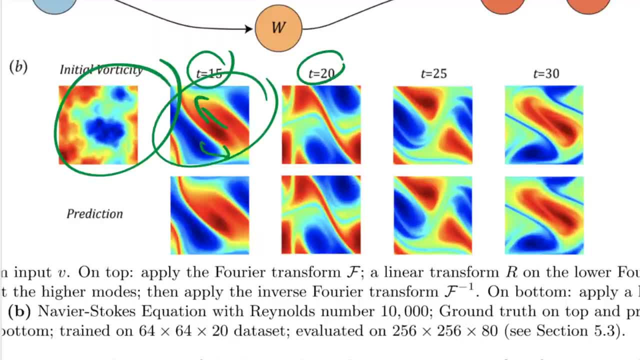 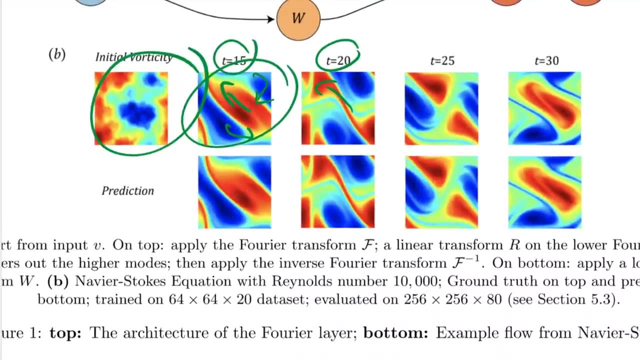 And see, this moves here, this moves here, And then at time step 20, you can see they are fairly moved. Okay, this blue thing moves in here as well, And they just sort of mix. And there's this. there are certain parameters that make the fluid more sticky or not so sticky, And the interesting regimes is, I guess, when it's not very sticky, so not not too sticky, but also not not sticky enough, And then these really complicated patterns occur. 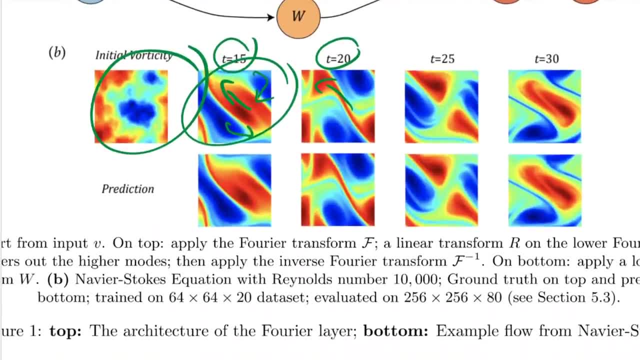 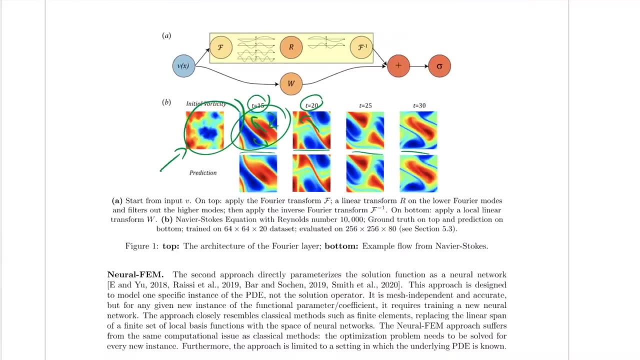 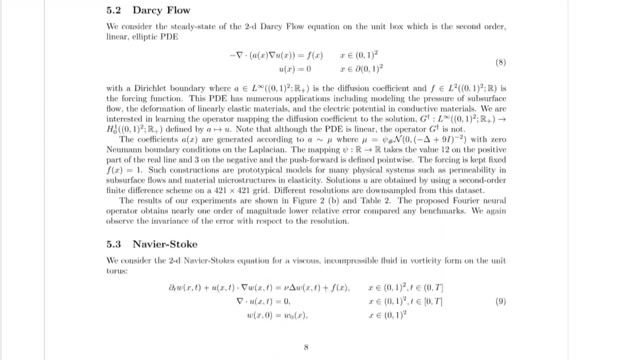 And to predict them would be very, very valuable. So you want something that takes in this initial state right here and outputs all of these, these future states, And usually this is done by these classical numerical solvers. So the Navier-Stokes equation is described by a set of partial differential equations, And you can see this down here. So Navier-Stokes 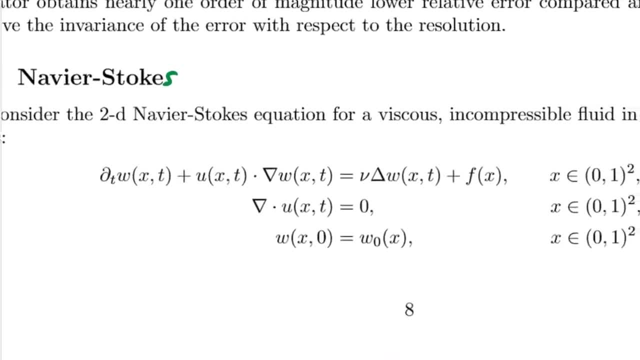 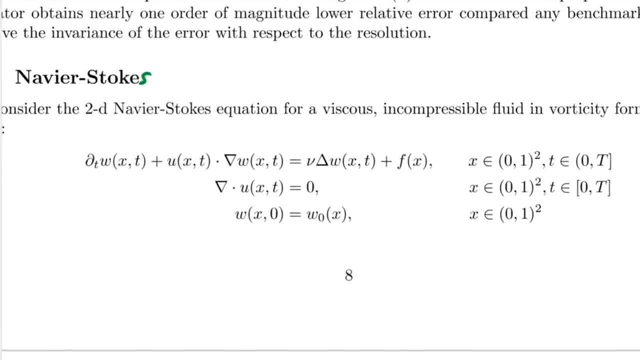 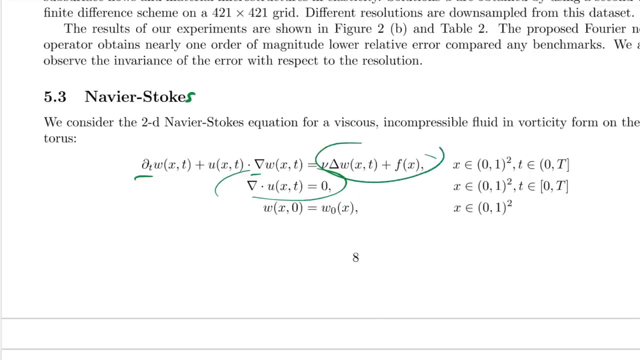 equation is described by this set of equations. right here is there Yep, And you can see that the, that this, this is fairly complex. it includes partial derivatives, gradients and so on. So this is the, this is this complicity, And it includes that on on both sides, And this is this, the. yeah, this is two derivatives, And then you can see that it's quite complex. 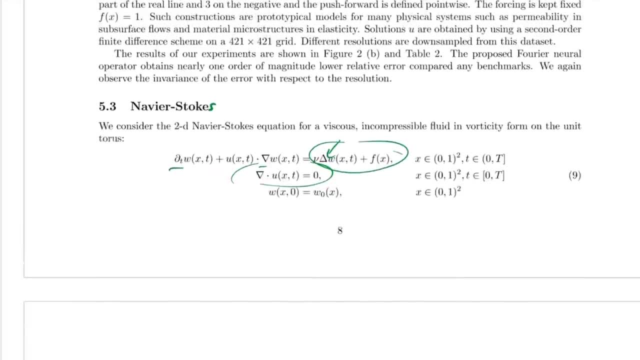 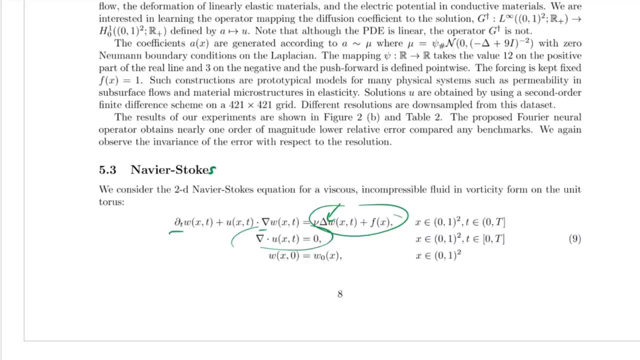 derivatives maybe, Or is it just the delta? I don't even know. I'm not an expert in partial differential equations by any means, So anything coming from that direction don't take me for granted. I'm going to give you sort of the thing of what I understand from this paper. 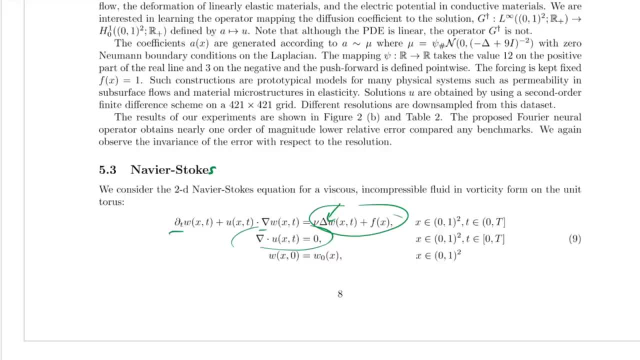 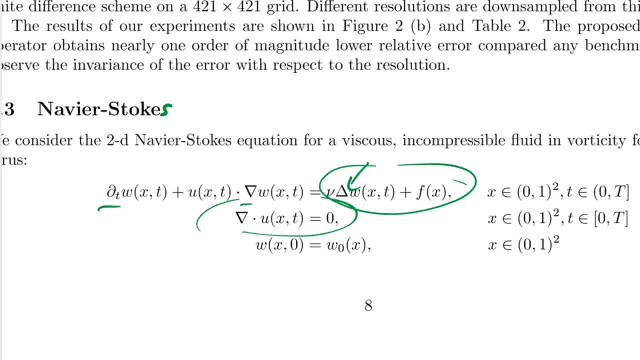 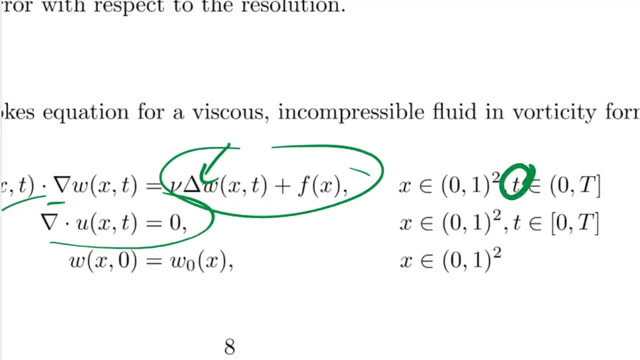 And so, with respect to that entire area, I'm not an expert. I just can understand that this is fairly complex And what you usually do is you take the initial state And you just evolve it in time. So you, you take this time parameter and you do, you go one little little time step. 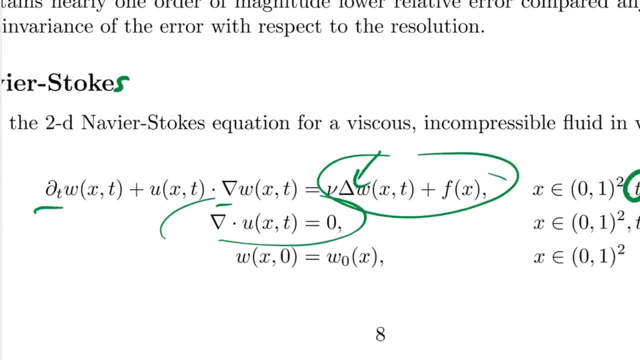 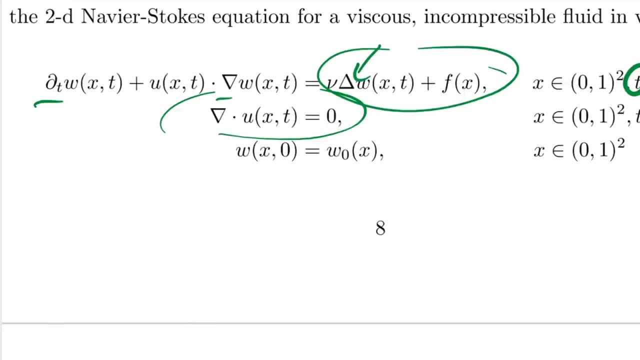 And then you calculate, because these are all sort of linear, linear equations. you calculate this one little time step into the future. you update your state, right It's. it's sort of like you know you have your points here and how they move. 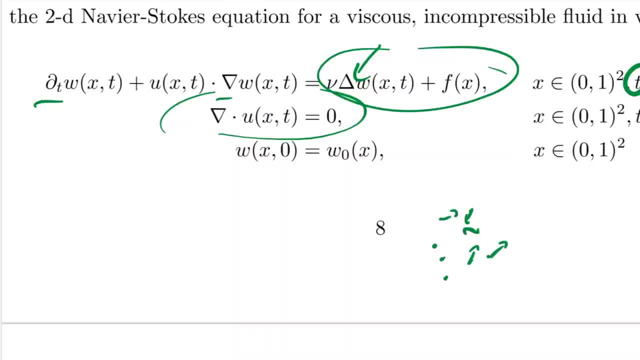 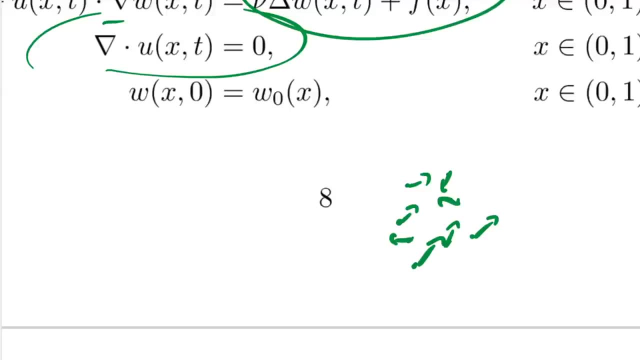 And how they move is given by their gradients. So these are all sort of linearized things. Now you don't want to move them too much per time step, Because ultimately, if this thing moves and this thing moves, then the movement of this arrow will change, because this thing over here 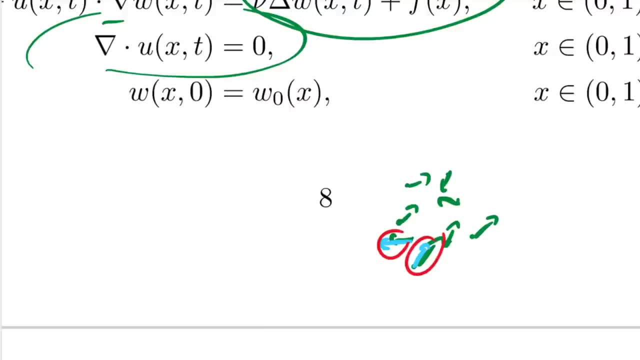 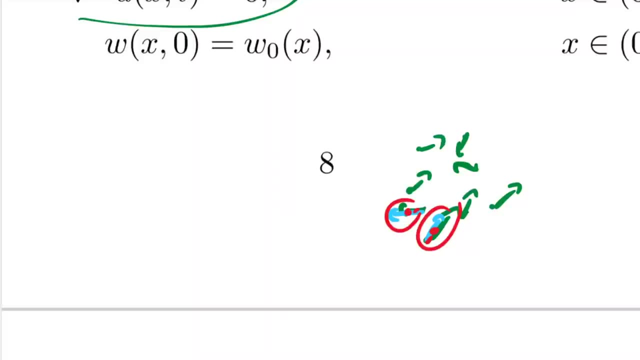 moves right. So you want to compute this one little time step into the future, like to here and this to here, And then you want to recompute all of these arrows. So maybe now that points a little bit more here, and that points a little bit more here, And then you want to. 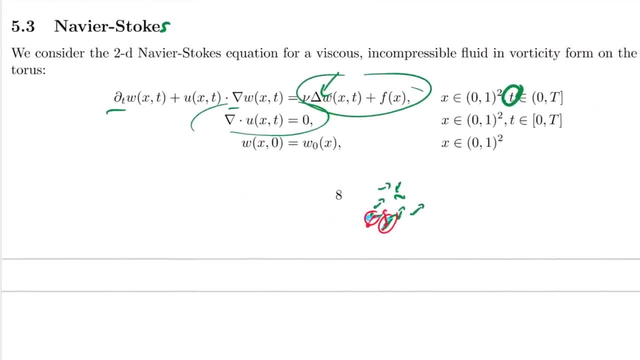 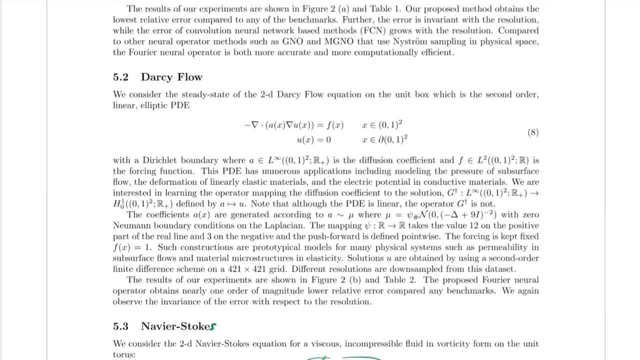 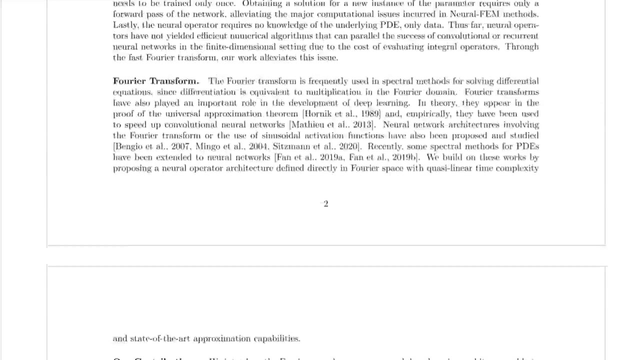 update it again. So you have these sort of these, these numerical solvers that go little tiny time step by little tiny time step. it's not even these. if here, if you see, t equals 20, or something, it's not 20 time step for these solvers, But these usually go like 1000, or 100. 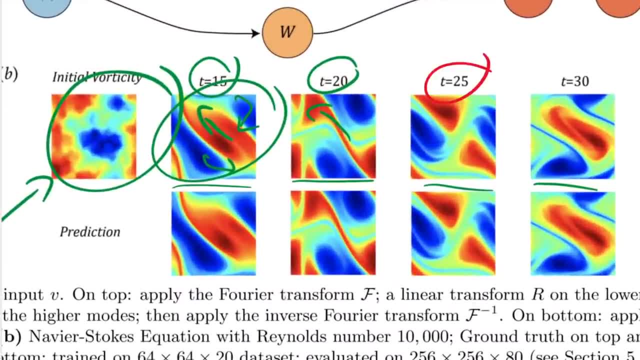 steps per time step, that is here, or something like this. they need to take very tiny steps to be accurate, And that takes a long time. So the idea is, can we simply, can't we simply simply input this, let's say this thing or like something at time 15, and directly predict? 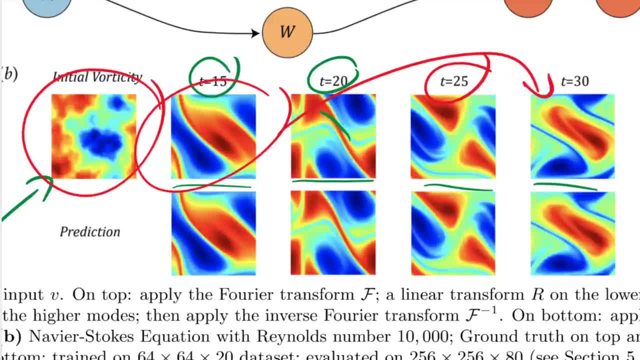 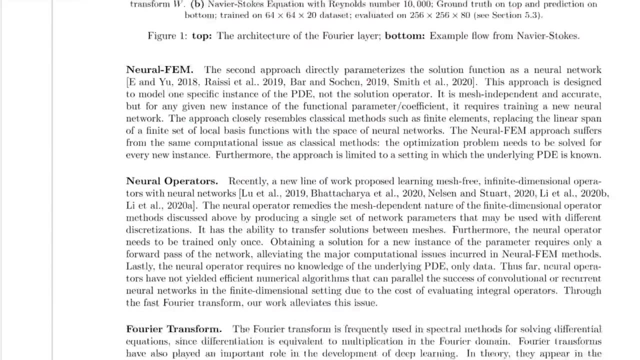 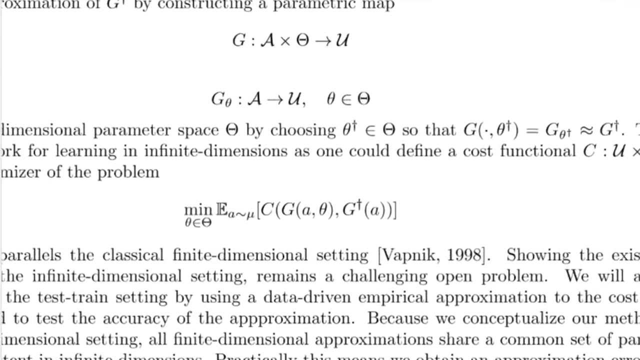 the thing at time 30. And that's exactly what this paper does, And a lot of papers have done this before, but without much success. So this paper proposes to do this in the Fourier domain and we'll see the path that they take right there. So they go into the will shortly go into, sort of 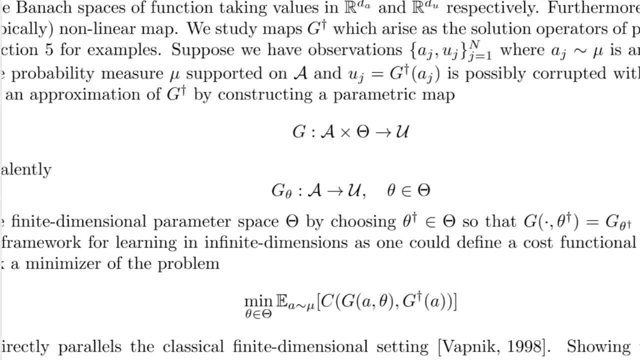 the basics right here. So what you want, what you're looking for, is a function g that takes an A and gives a U. So what you're looking for is a function g that takes an A and gives a U. So what you're looking for is a function g that takes an A and gives a U. 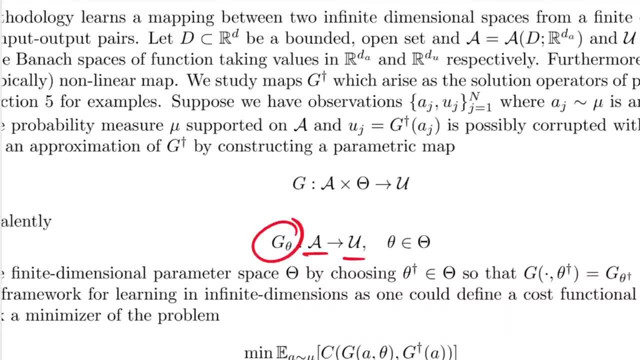 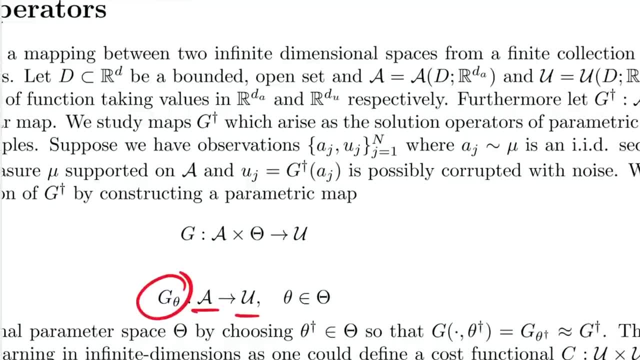 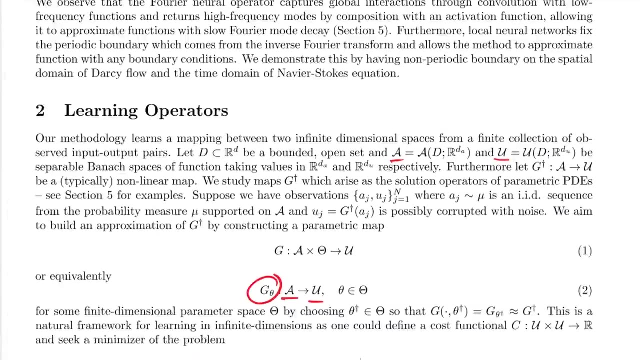 So what are A and U? A and U are both function spaces, So A, A and U here are functions. So A is a function. as you can see, A is a function and U is a function, but you can characterize them as data points. So in this, in this way, there is a functions and data points are sort of interchangeable. you can see an image like this as a data point. 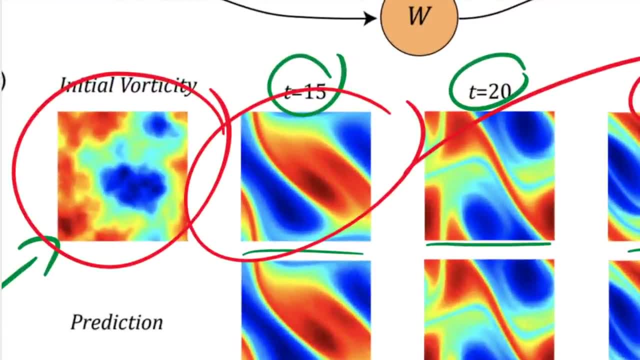 like this as a data point, Like this as a data point Where it's an image, but you can also see it as a function, where every x and y coordinate is mapped to a value, right? So when when they talk about functions, very often they talk about this type of function. 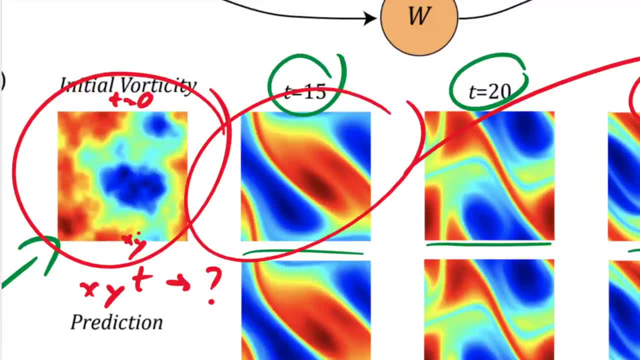 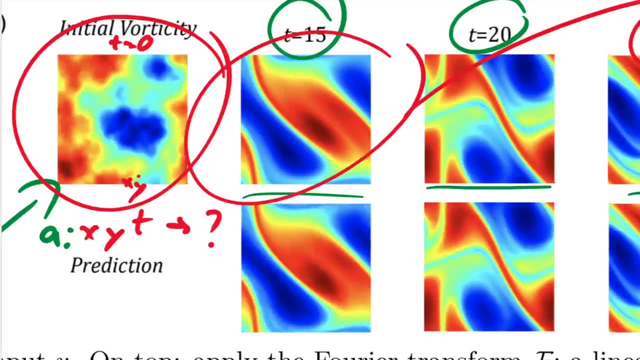 Where you have x, y and t. t is also. t is zero here, X. So the function would x, y, t. map that to some value. Right here the vorticity values are inside y or 0. And you want to transform this function. So this function would be a, a would be the function. 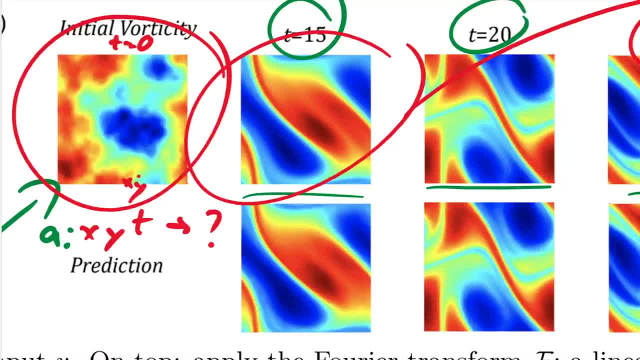 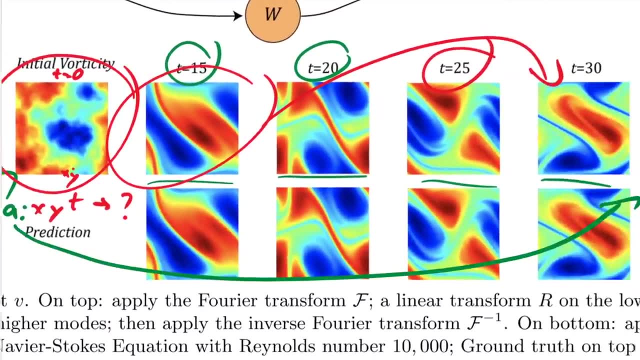 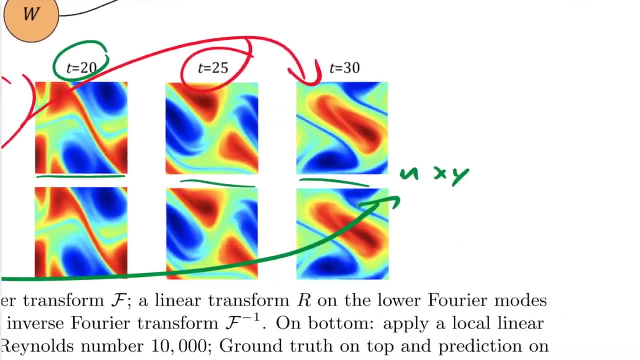 at time. let's say zero or something, or times zero to 15, you would want to map that to the function, the function u. that also takes an x and a y. let's leave t out for the moment. that also takes an x and a y. and let's say t, but t is set to 30. And maps that to a vorticity. 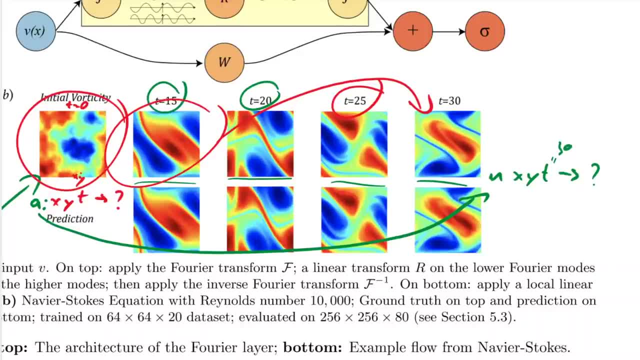 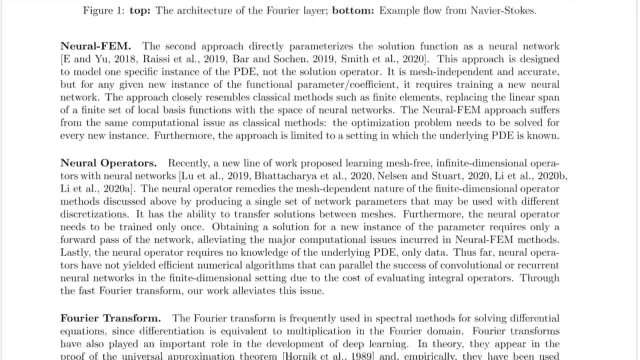 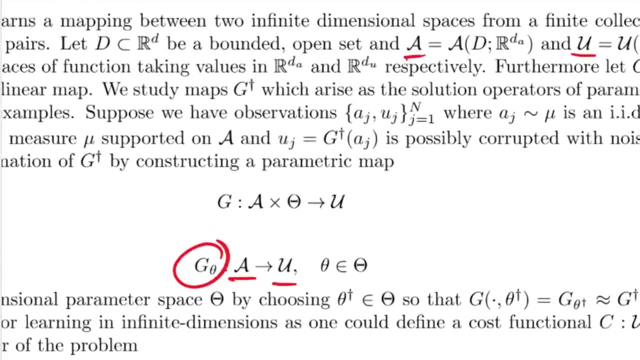 right, So you want to input a function and output a function, but it's the same as inputting an image and outputting an image in. as for from an engineering perspective, of course from a math perspective it's a little bit different, But other than that it's a fairly 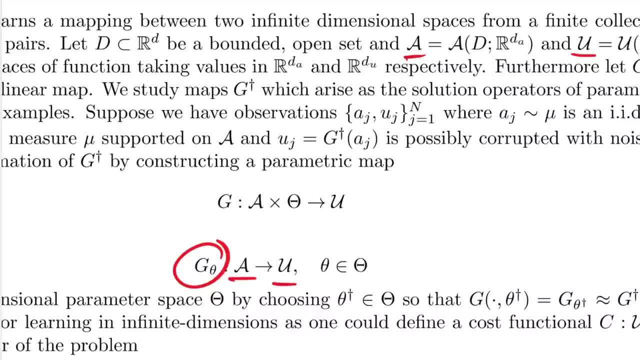 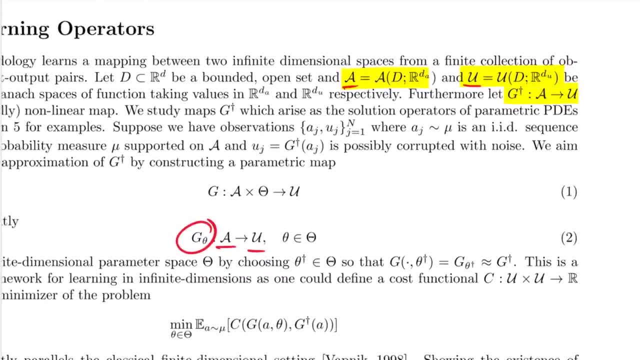 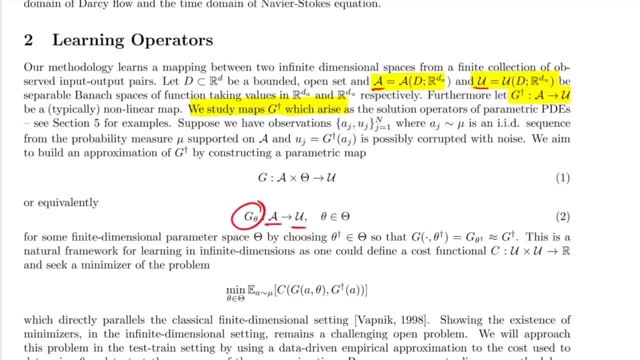 standard machine learning problem. So you have this, these sets a and u, And you're looking for this function g that maps a to u. Okay, so we studied maps which maps g, which arises the solution. operators of parametric PDEs. 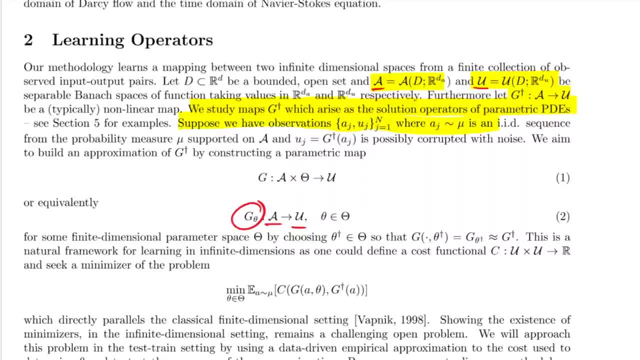 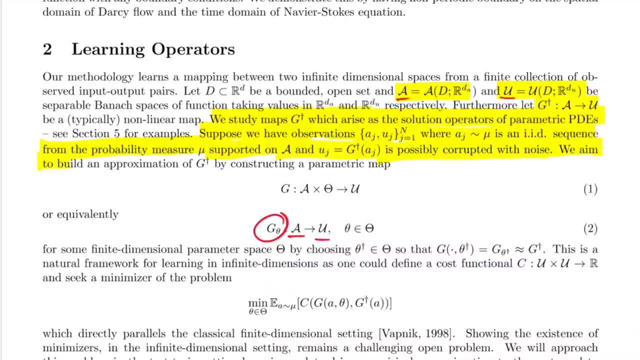 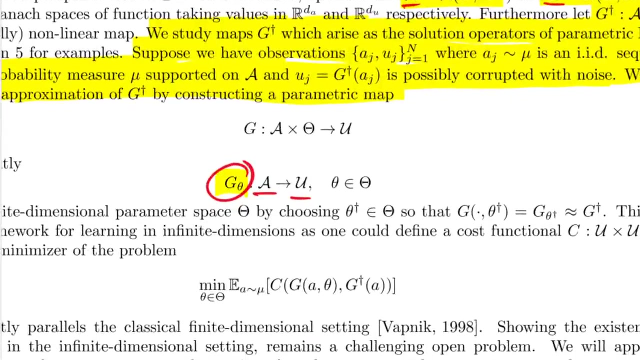 Suppose we have observations where a is an IID sequence from probability measure mu, supported on i And u is the a transported by g, it is possibly corrupted with noise. we aim to build an approximation of g by constructing a parametric map. this g right here. So it's a bit of a mathy. 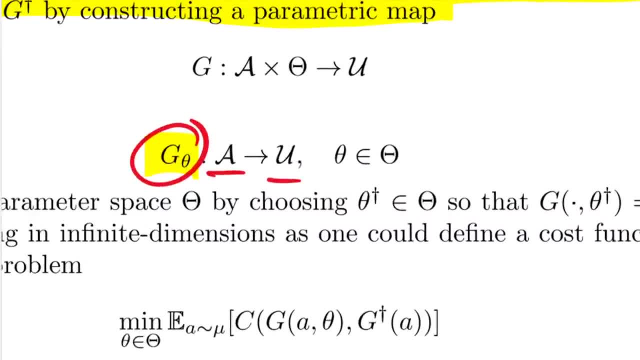 way of saying. we have a bunch of data points where we were: a- this is the initial state- goes to u, which is the state at some point in time, And we know that there is a function g- this is this g, with this inverse cross, we know that there is a true function that maps any a to 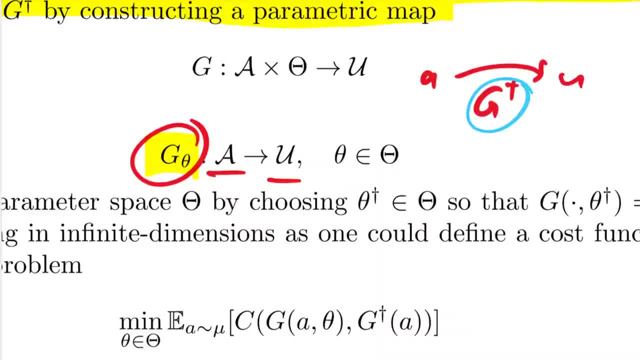 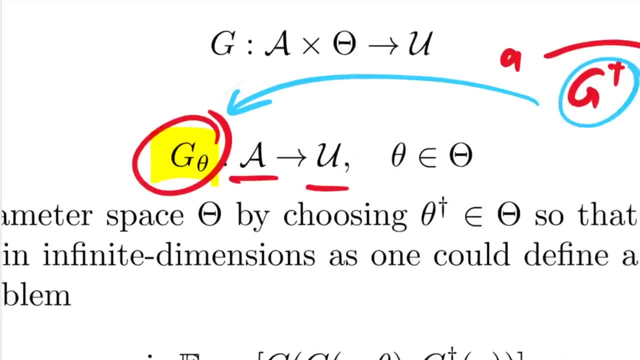 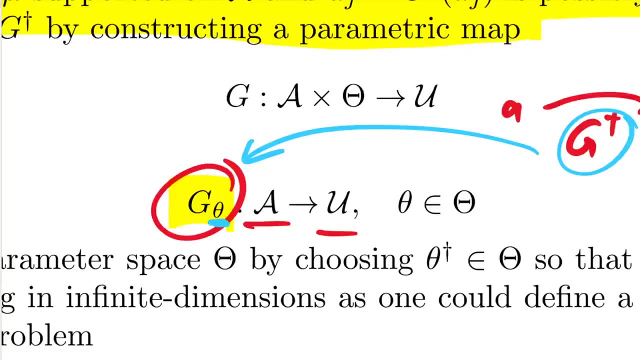 u. So a single function, g, that can, if I input the initial state, can give me the output state, And what I want to do is I want to approximate this by a parametric version. So these here are the parameters And, of course, as you can guess by now, g is going to be this. g right here is going to: 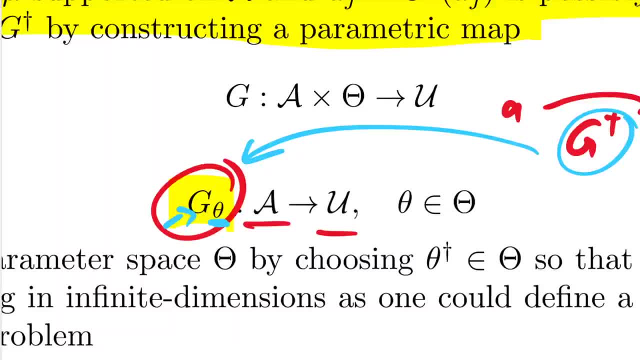 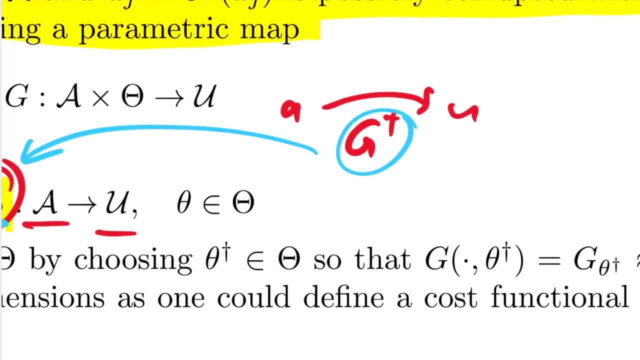 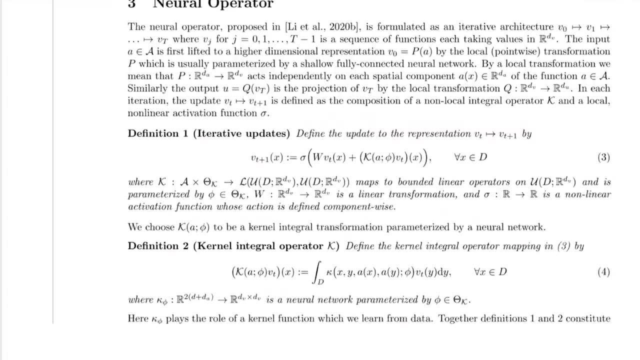 be a neural network That is parameterized by theta. So these would be the layers of the neural network And we're going to input a into the neural network and we're going to get out u. So that's basically that there is quite a bit of math right here, And the math here is to derive what they call a neural operator. 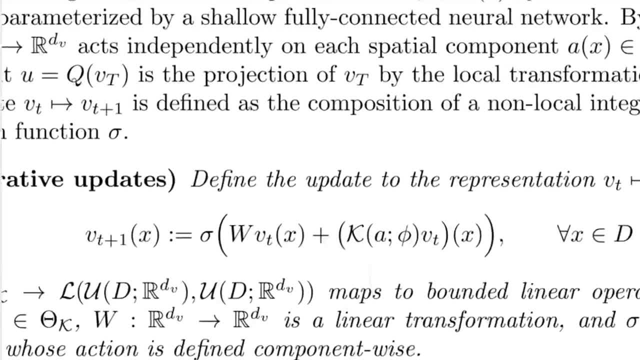 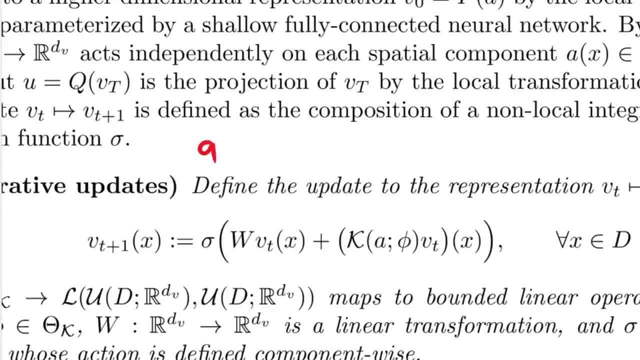 So here is one layer of this neural network. As we said, we're going to input a. now, a first thing that we do: a is going to be, let's say, up projected. So a is going to be made into a latent. 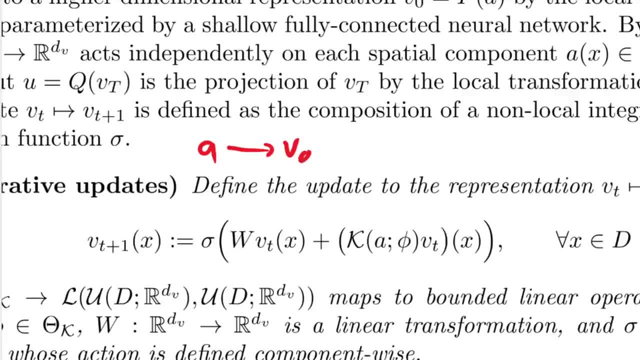 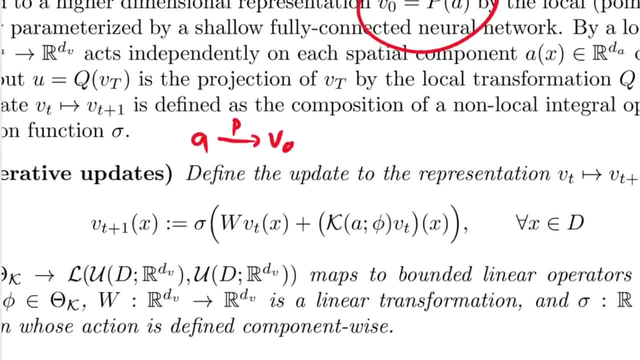 representation v zero. So this is- let's call that here- p. So there is a function, p, which is going to be a little layer of neural network And it is going to produce this v zero. So v zero is going to be a latent state of the neural network. 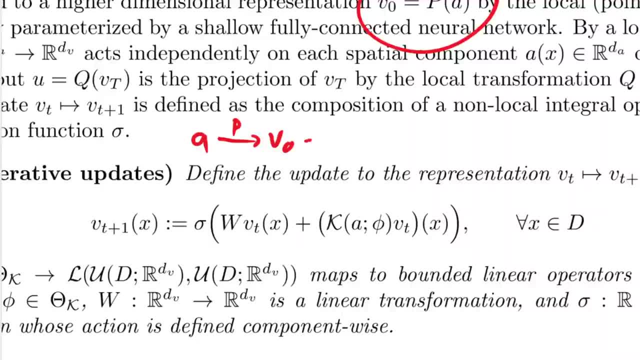 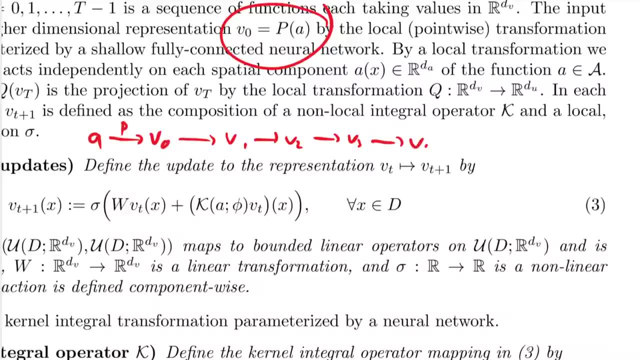 neural network And then there is going to be a number of these layers that transform this to v one, v two, v three And v. I think there are four layers of these in their particular implementation, but there don't need to be four layers. you can choose that, as you can choose any depth of neural. 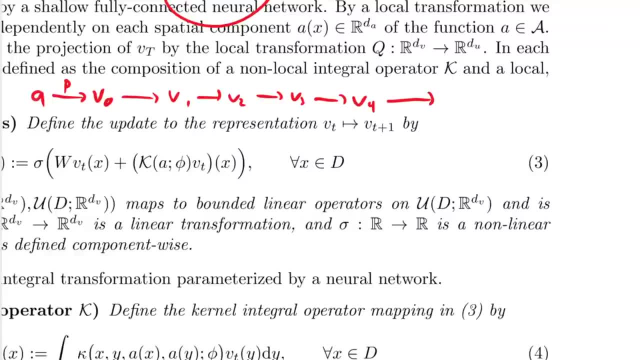 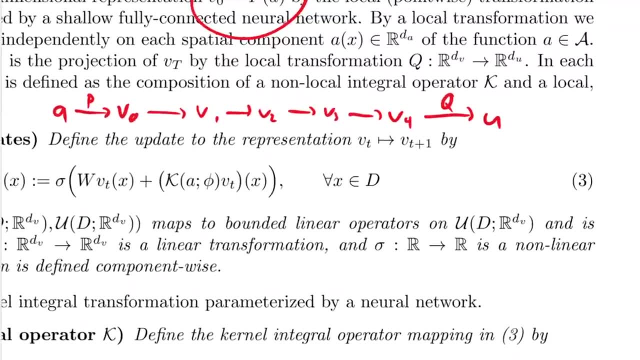 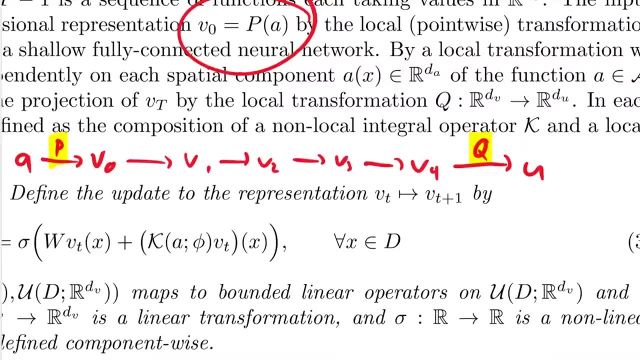 network And then at the end you're going to project that down to whatever output you want. So that's going to be V? u. Okay, so this function here is called q And these are just going to be neural networks of p and q are going to be your very, very classic up projections and down. 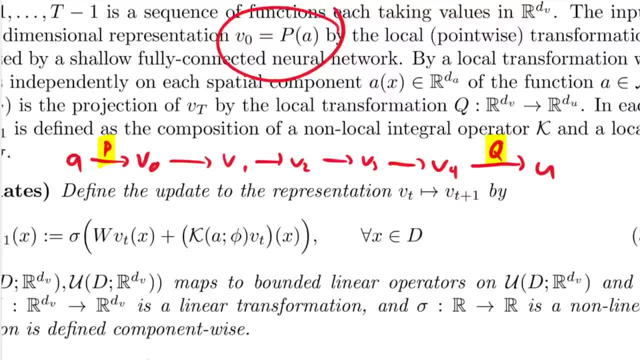 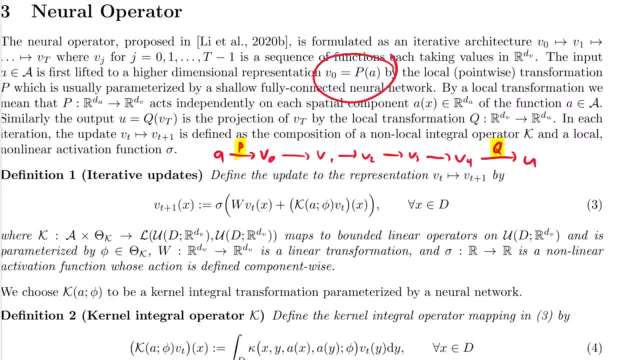 projections of data point. we'll get into actually. we'll get into sampling. Let's go actually right now. So So one thing right here- and they stress this- is that they work in function space, right, They? they don't. 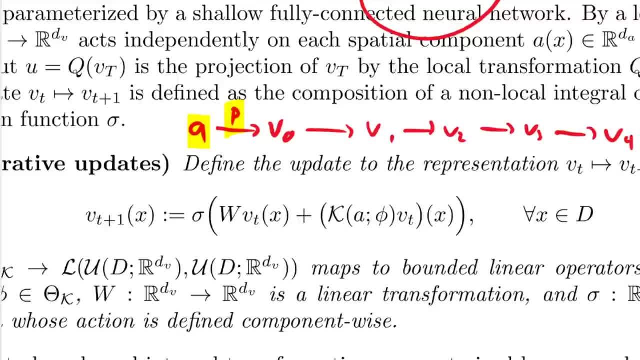 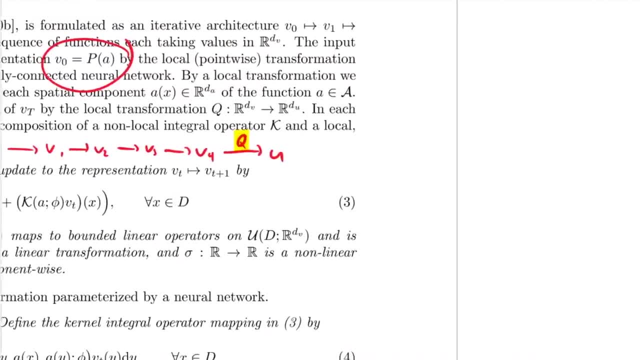 they don't work on a function space. right, they, they don't. they don't work on a function space, on the, let's say they don't map the data point to the data point. what you could do is simply have like a convolutional neural network and image to image network and so on. But what is the problem? 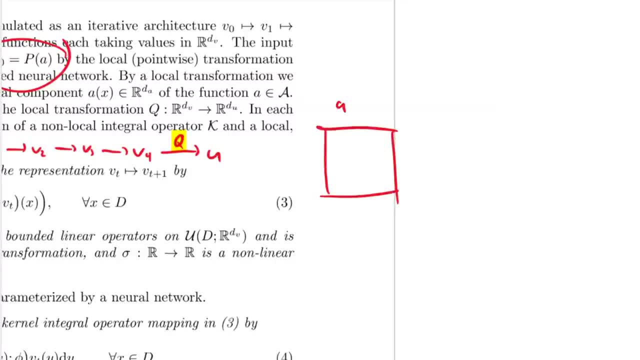 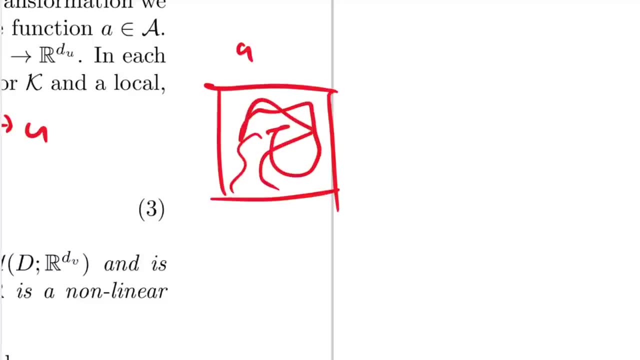 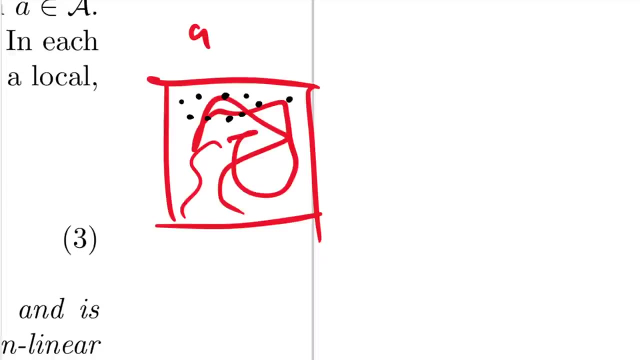 with that. So if you have your a, which is your initial state and it has, you know it has these bunch of fluid things right here, And what you do when you have an image is you sample this, right, you sample this. a different- sorry, maybe a regular grid- I am terrible at regular, So you sample this. 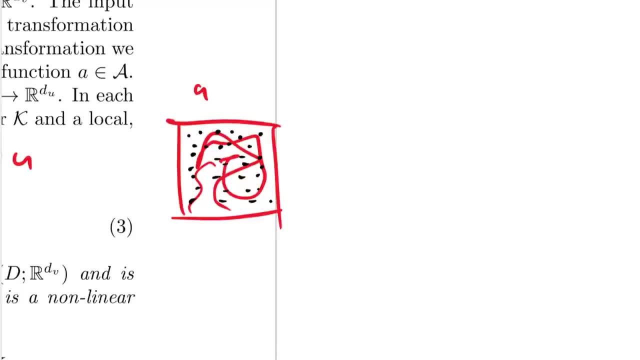 into a certain amount of pixels and your neural network will operate on this right. this will give you some kind of a tensor which is, let's say, we have a, so this is a seven by seven grid. okay, so your neural network is going to expect this as an input dimension And whatever you as 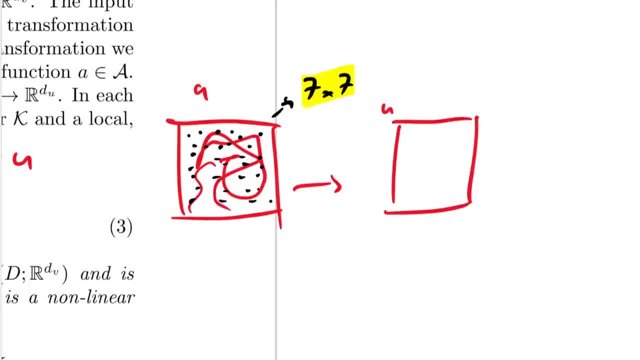 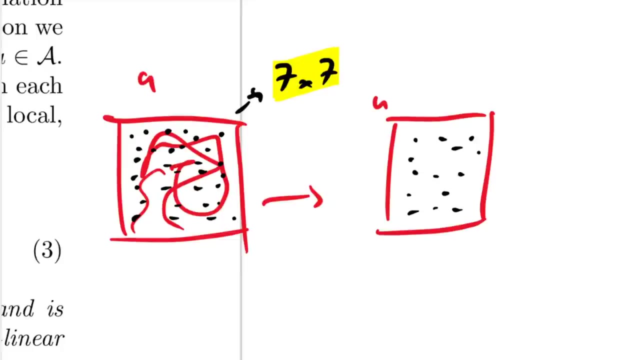 of course. so you map this to you, which is also going to be some sort of image, okay, where you need to output pixels. So again, you have some set resolution and your neural network can only operate at that particular resolution. What they're doing right here is the cool thing about is it can operate. 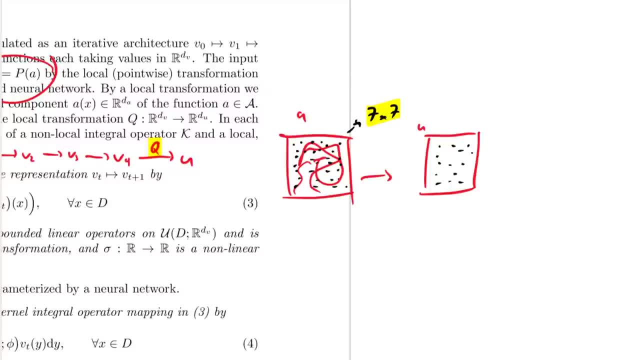 at any resolution. So once you've learned the network, you can input higher resolution images or you can output higher resolution images any, any sort of image, And you can deal with more resolution, less resolution, sampled irregularly. you can. 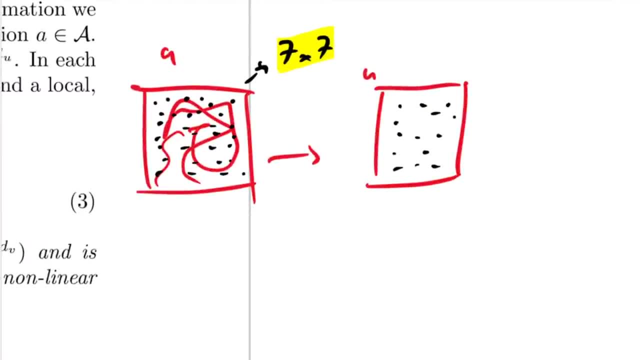 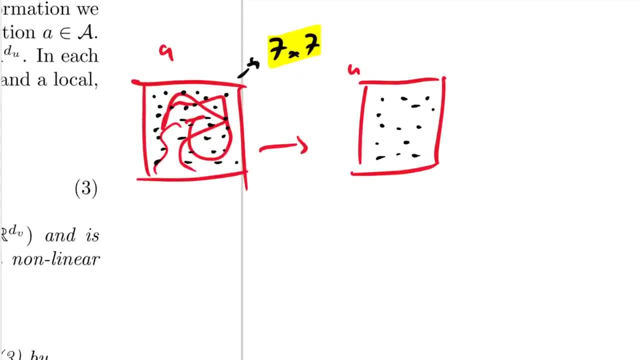 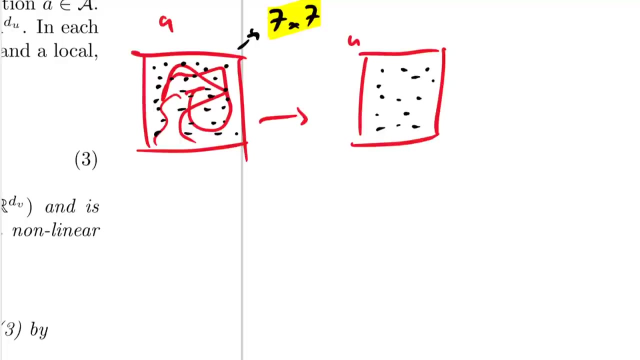 deal with a lot of things once the neural network is their neural network is learned. And how do they do it? They do it by only ever acting pointwise in the spatial domain. So what they're going to do is they're going to take this a, and now we get into the more critical things. So here a and u. 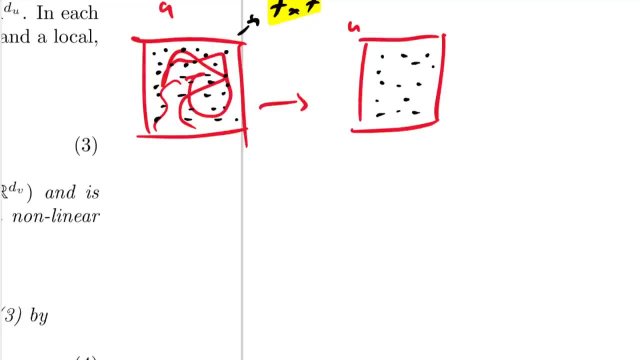 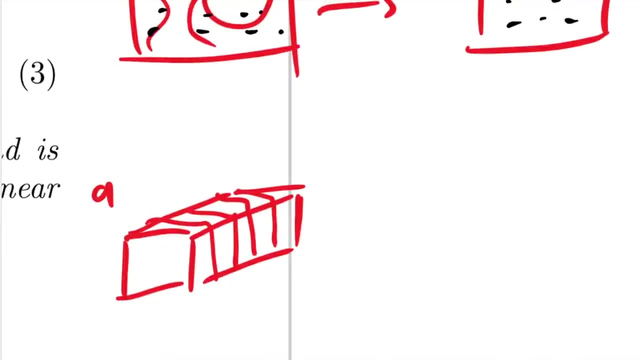 the beginning state and the end state. In fact, in this Navier Stokes example, a is a tensor like this. So a is going to be a tensor with slices And each slice describes one time step up to a given time. So this here could be: t equals zero, So there is kind of the initial distribution. 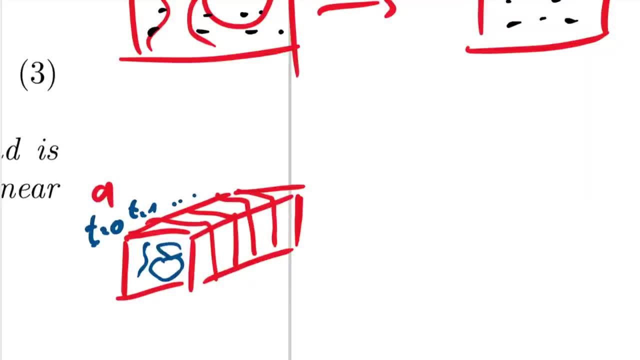 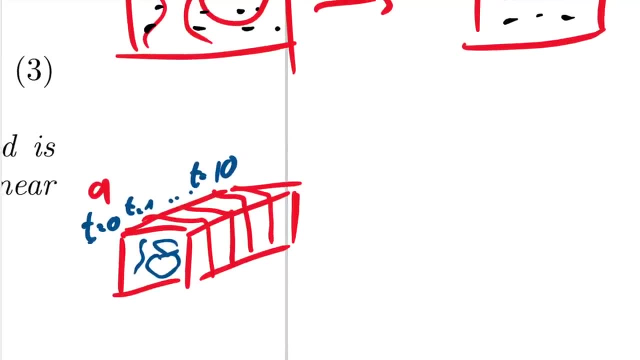 and then t equals one, and so on up until t equals like 10.. Let's say I think they do 10.. So if they let this thing evolve for 10 time steps- and I'm going to guess they do it using 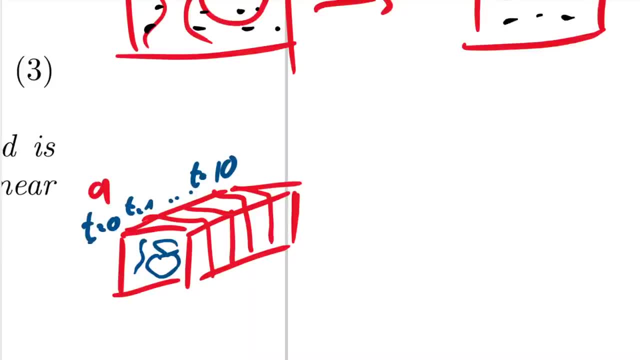 one of these classical methods And that's the input. So the input isn't just the initial state, the input is actually. here is what happened in the first time: 10 time steps. And then the output isn't just at the output at some particular time, But the output is actually. 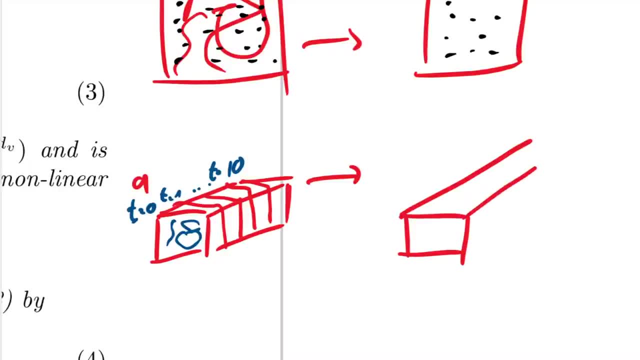 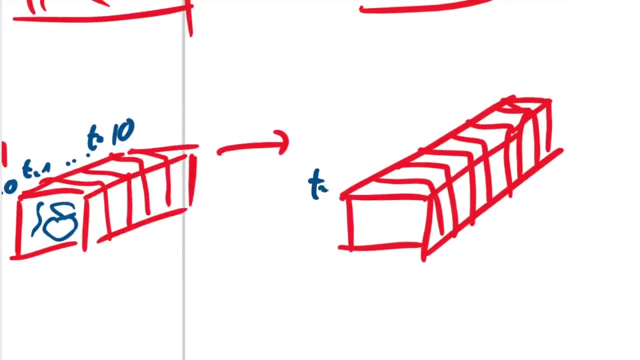 also a slice right here. Sorry, a sliced tensor, So each slice here describes the output at a particular time. So this would be: t equals 11. Up until t equals 50.. Okay, so this is this is you. So the top one is sort of the conceptual. 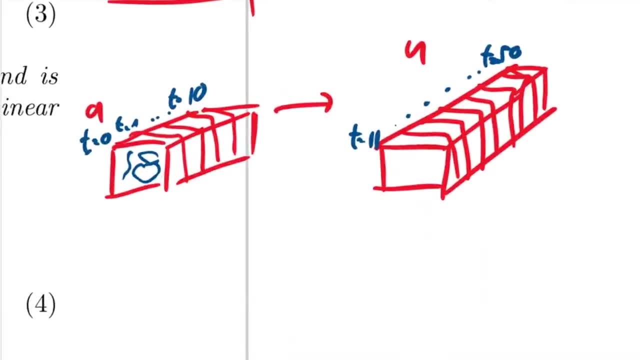 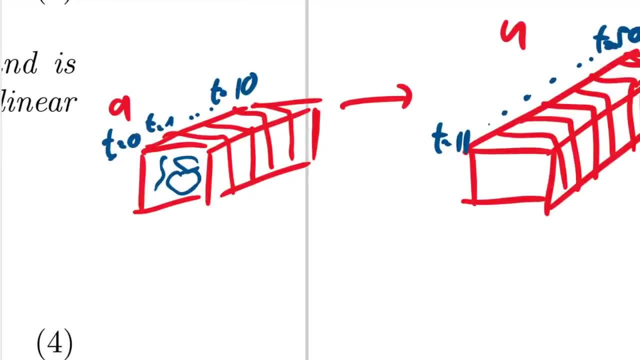 thing, But the bottom one is what really happens. So they input 10 time steps and they get out the 40 subsequent time steps. they predict them all at once. Okay so, and now you can see that, in this particular case, how I can understand this is at each pixel. 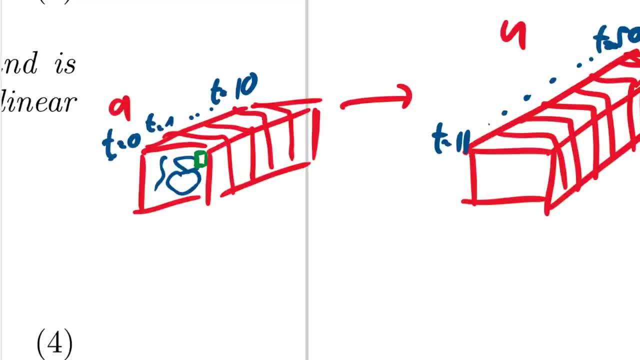 here. I want to know what. what is that pixels value? after what? after like certain amount of time, steps okay, like 11, or 50,, right here, or 40. And of course, the result is going to not only. 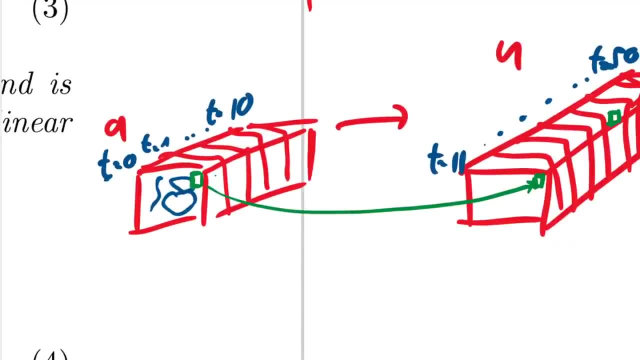 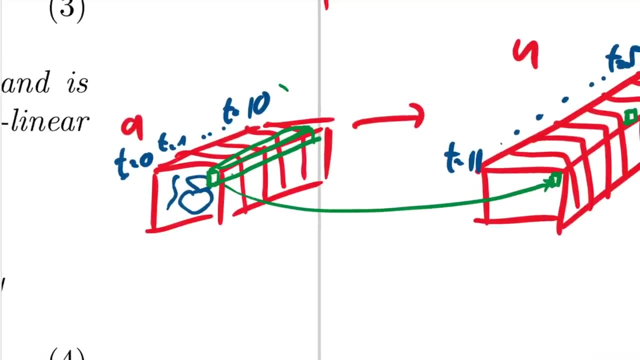 depend on the time zero, but on the entire evolution of time zero to time 10.. So this here is an entire column For that pixel And this is akin to that particular pixel having this many channels. So here I can just say: well, these are technically 10 channels or 11 or something like this. I probably screwed. 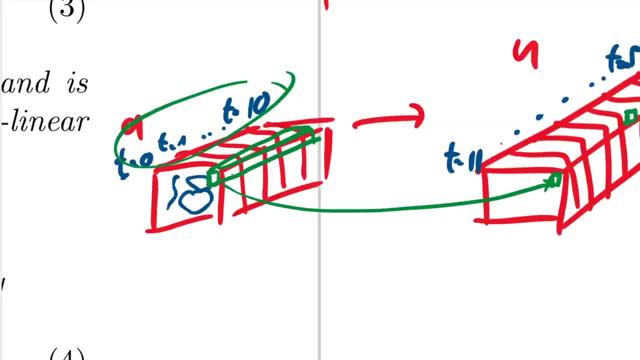 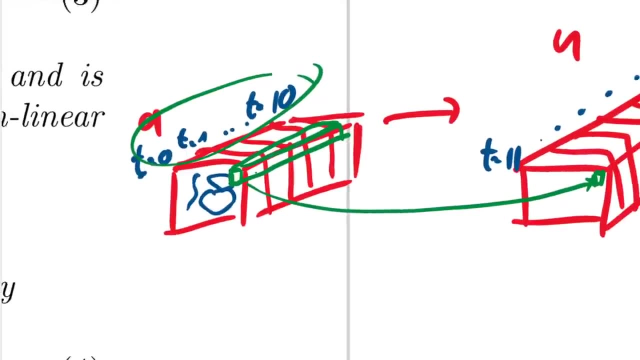 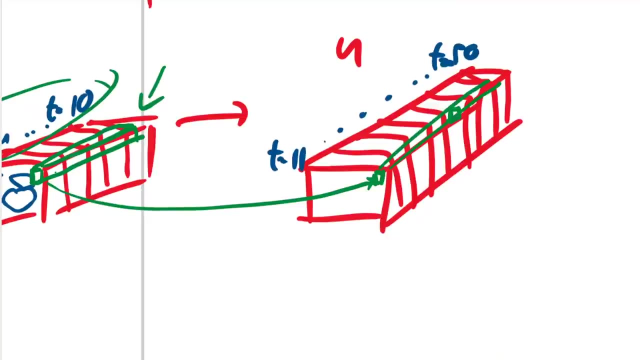 up this should be: t equals zero to nine, and then 10 to 49.. But so this is. this is an entire stack. this is, we can interpret this as input channels. right here, interpret these as output channels. Okay, so ultimately, one pixel is going to have input. 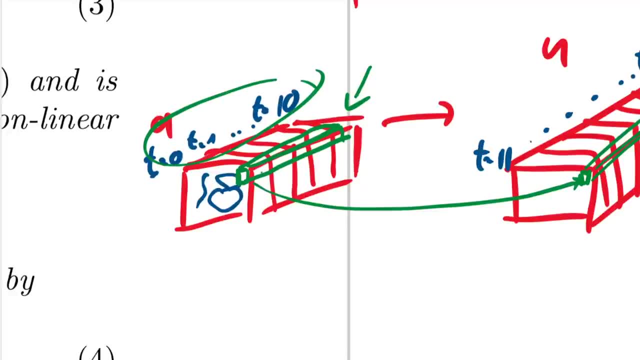 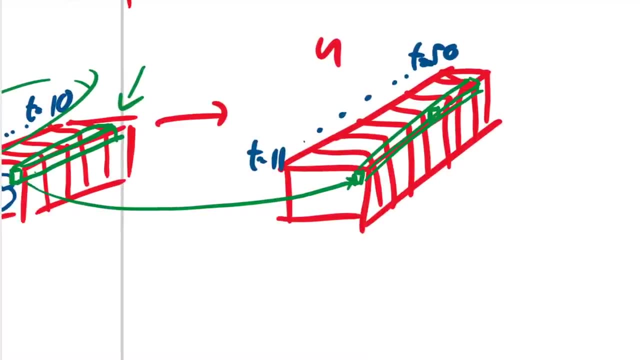 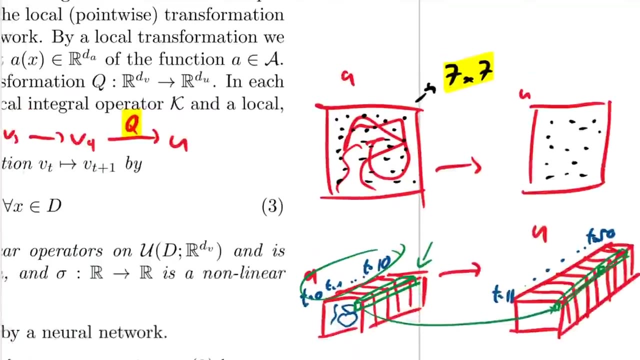 channels, all the time steps that happened up until the point where we want to predict and the output channels are going to be at the same time, all the time steps of what we want to predict. Okay, So these projections. now coming back to this, they simply work in the channels. 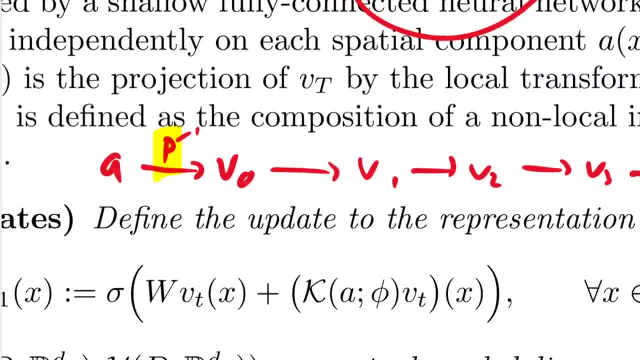 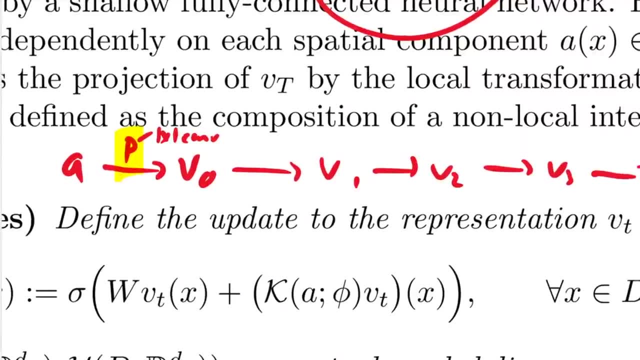 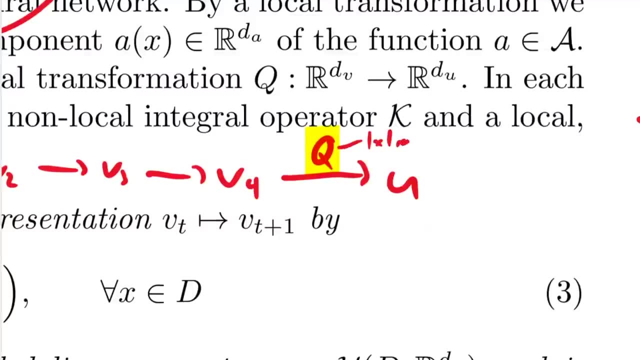 So these P and Q, they are one by one convolutions And the one by one convolution simply up project and down project. These features, you see, these are one by one convolutions. Actually they could be dense layers. Let's check that in the code. 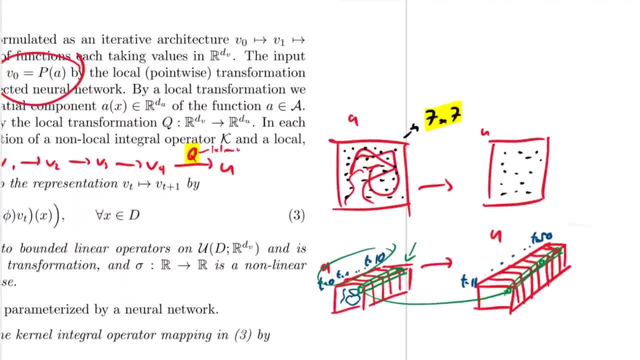 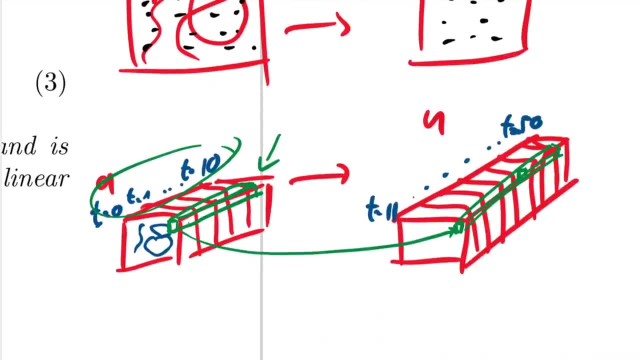 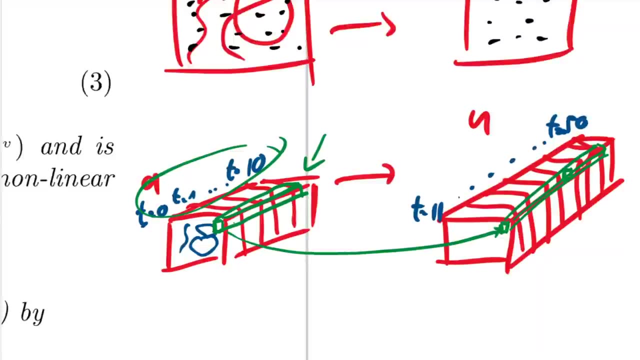 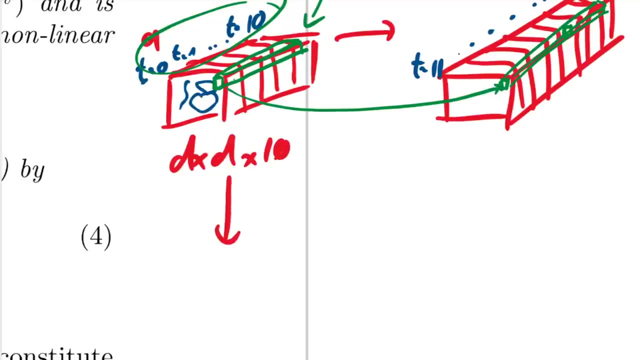 Later. But for sure, what they do is they only work pointwise, So they don't. they don't mix the individual pixels together In here. you simply get at like a D by D grid with each has 10 channels, And then you simply up, project that to. so here you have D by D times 10. And then you up. 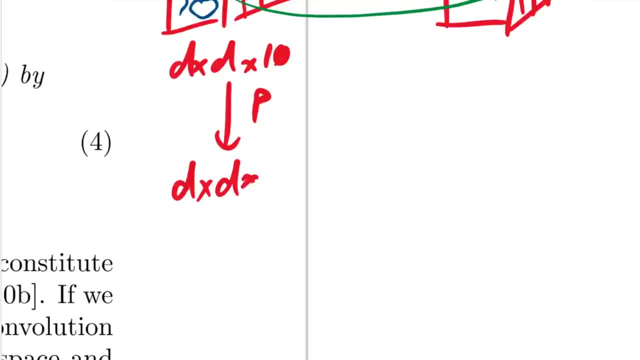 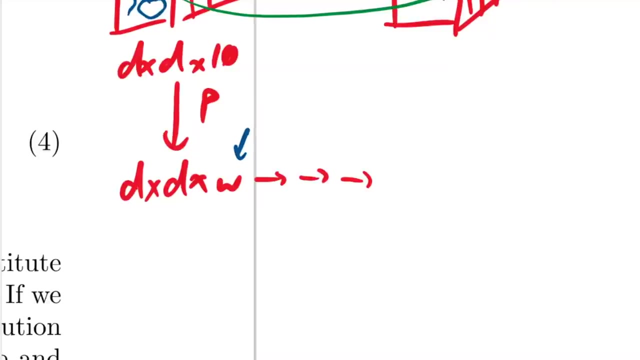 project that using P to D by D times, and here as a parameter that you choose. so this is sort of your latent dimension, okay, And you are going to transform this tensor, keeping it in this D by D, by w dimensionality until you back projected. 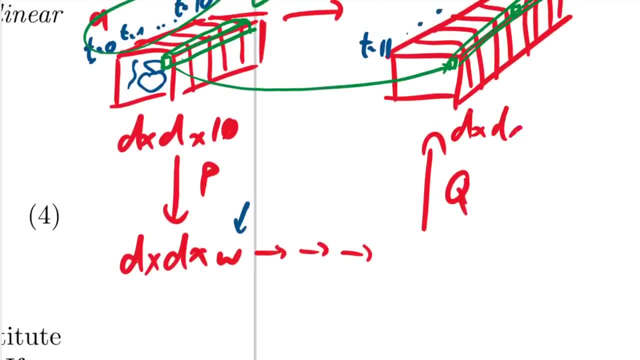 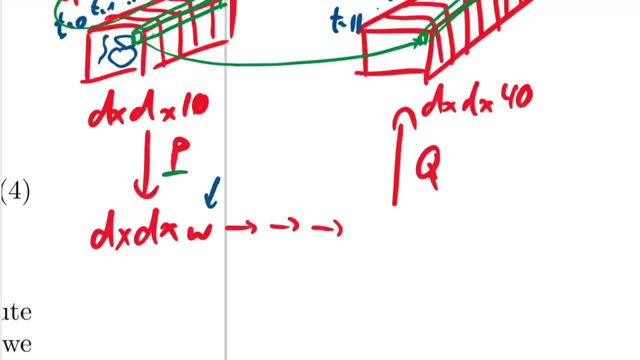 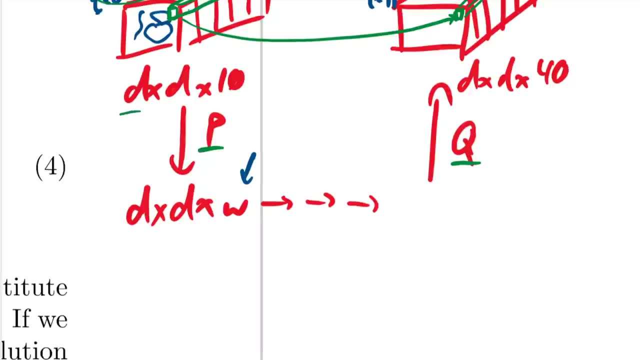 using Q to D by D, by, in this case, 40.. Okay so, but this, this and this, they only work pointwise, And that means there is no particular dependence on the D right here. So the next data point could. 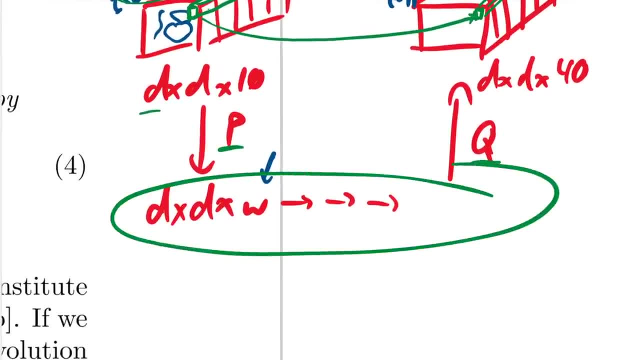 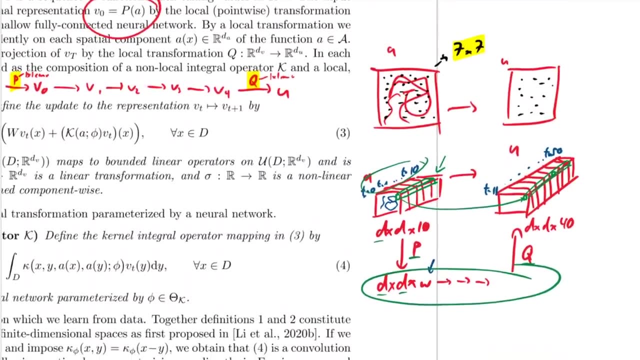 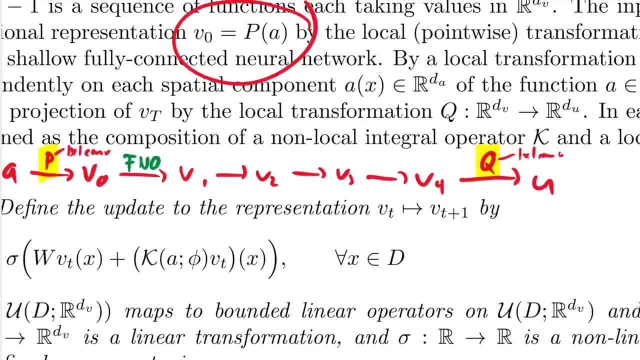 actually have a different D, as long as this pipeline right here can handle different dimensions, because the P and Q only act pointwise, you're good. So what do? what do these magic layers here do? So these are these Fourier neural operators. okay, they transform one hidden state into the. 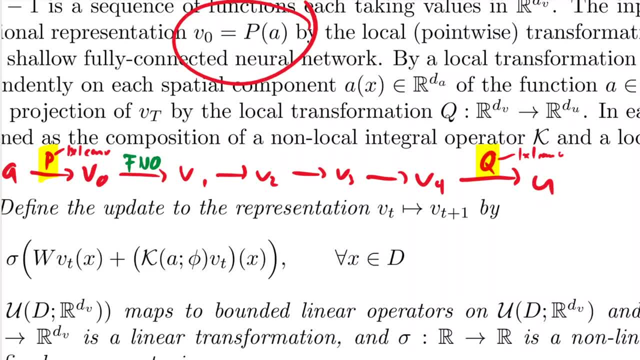 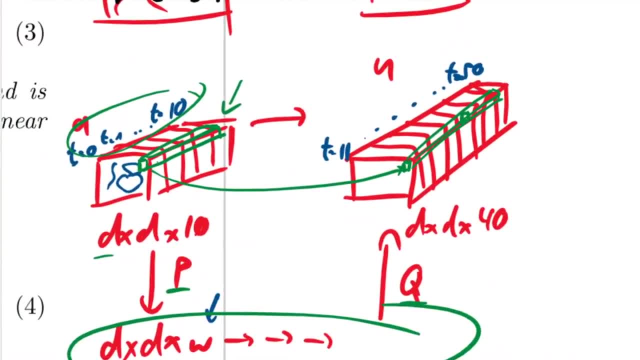 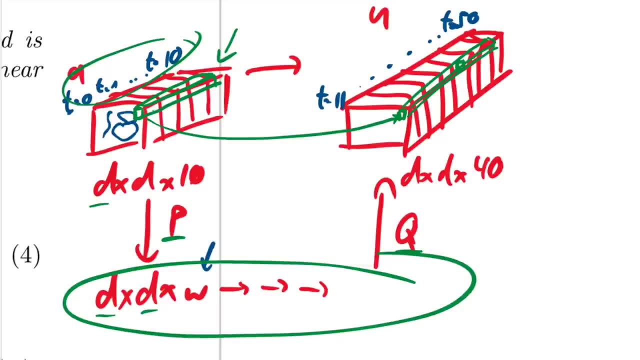 next, Note that we have four of these layers, So they don't need to be the same as the number of time steps. we're trying to predict, you see, And it's pretty clear from here. So we, these four hidden layers, they're simply transforming this entire volume right here, this entire input volume. they 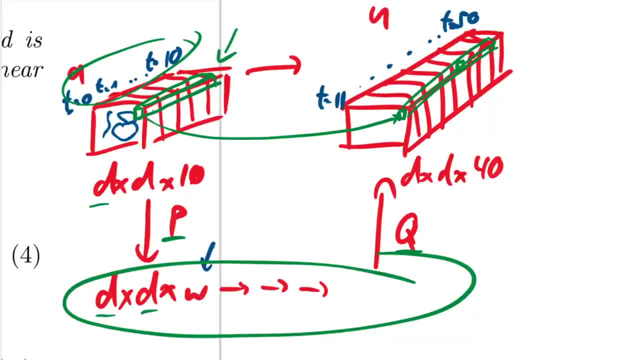 are transforming this as a sequence of latent states and then outputting this entire volume. So this down here has nothing to do with the time steps that we're trying to predict. it is simply a sequence of computations, of latent computations, And you know that in a neural network, the deeper 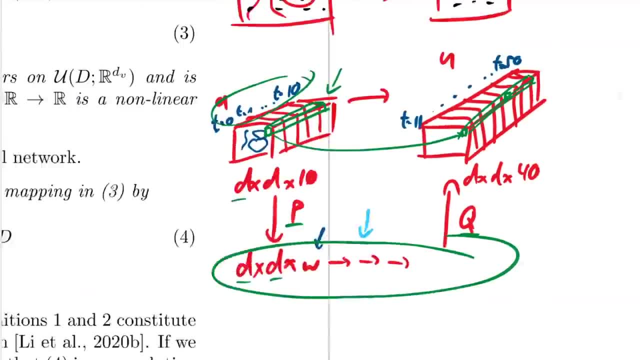 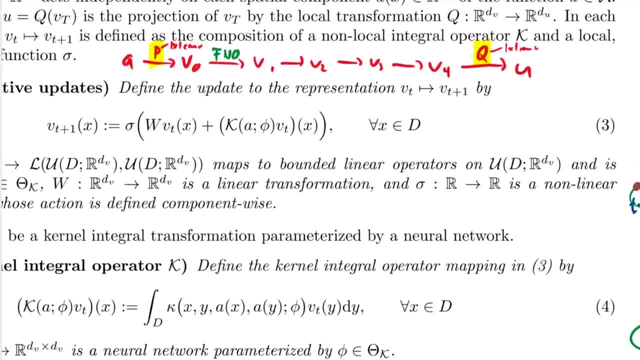 you make it, the sort of more complicated functions arise, even though of course the universal approximation theorem says that with one hidden layer you can do anything. But in general, if you have deeper neural networks, the more more you can kind of make more. 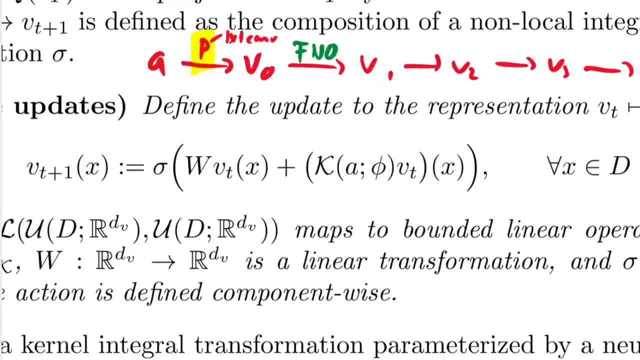 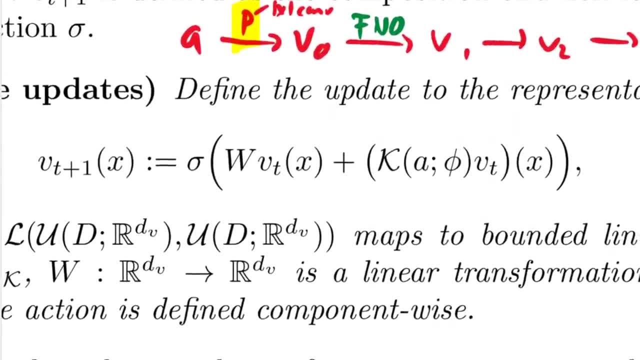 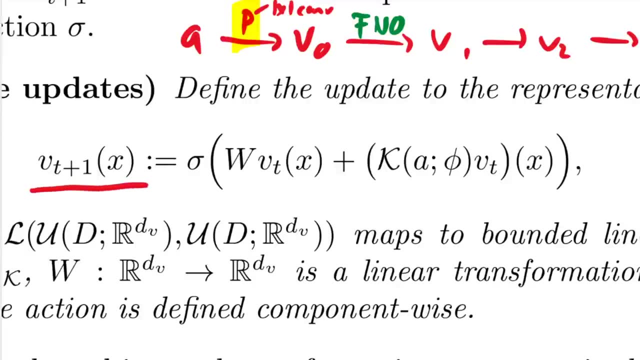 complicated things, And so four seems to be a good number of complicated for these particular problems. So here's what one of these layers does. It is very much like a residual network. So here you have v. the v is the hidden representation at t plus one, and t plus one is not, as I said is. 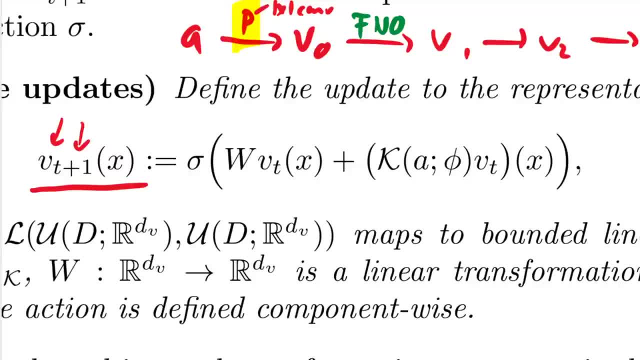